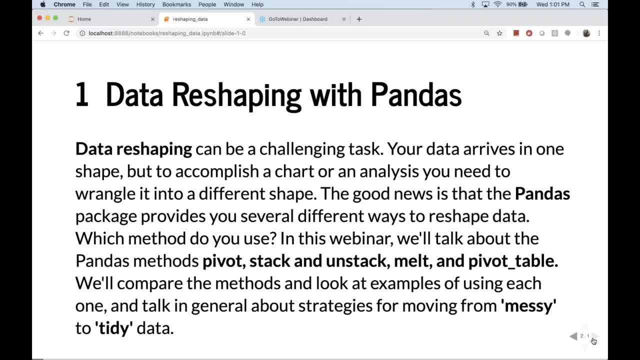 what are the differences between these methods and when do I use each one? And this is what this webinar will hopefully cover for you- Things like pivoting, melting, stacking and unstacking and the pivot table method. We'll compare these. we'll talk about some examples. 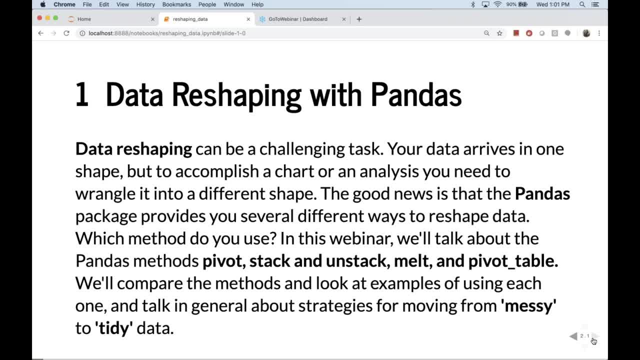 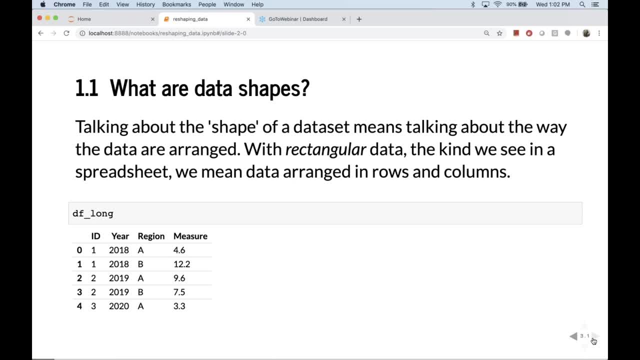 some differences between them, and then we'll talk in general about strategies for moving from messy data to tidy data. So first we just need a little bit of vocabulary to get us all on the same page here. What are data shapes? What are data types? What are data? 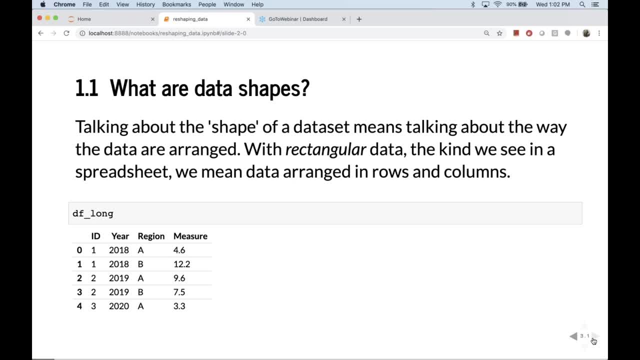 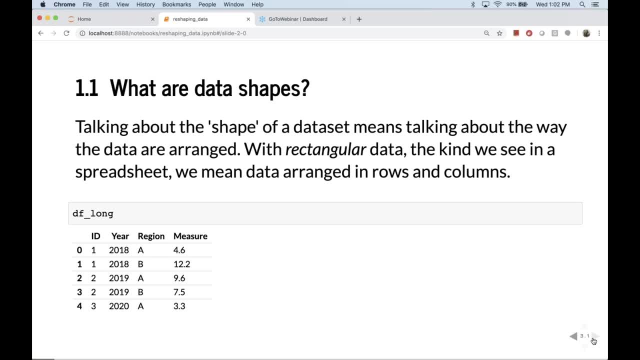 about in a spreadsheet. we mean data arranged in rows and columns. So here in this example, pandas data frame df-long- we have some data in rows and columns. We have the ID column, we have a year column, the region column and some kind of numerical data on the measure. 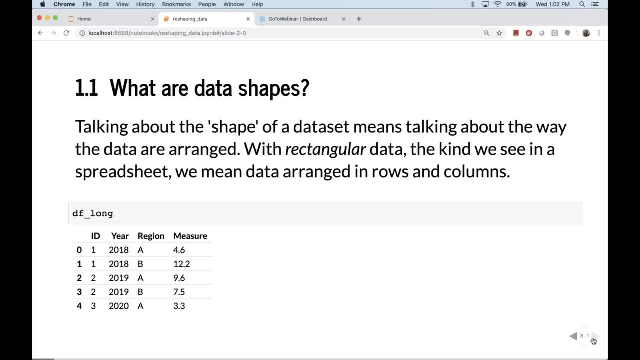 column And we can see that, And we can see that. Now, that's perfectly fine. That's one representation of this data, but we could represent it in a different shape, like this: So this is the same data, but rearranged in a different shape. 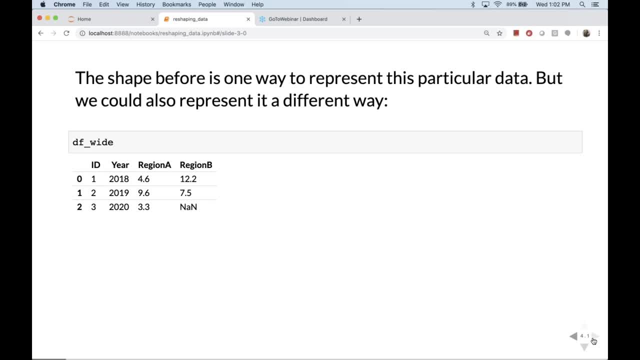 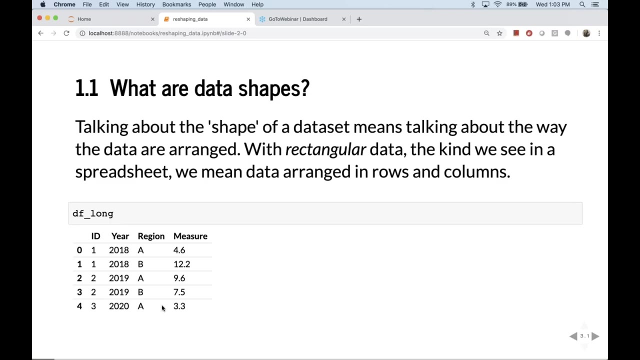 So we still- we see we still- have the ID column there. We have the year now collapsed into three values and then we have two columns for region A and region B. Again, we'll go back to the previous slide here. Just a glance at this. So here's the same data. 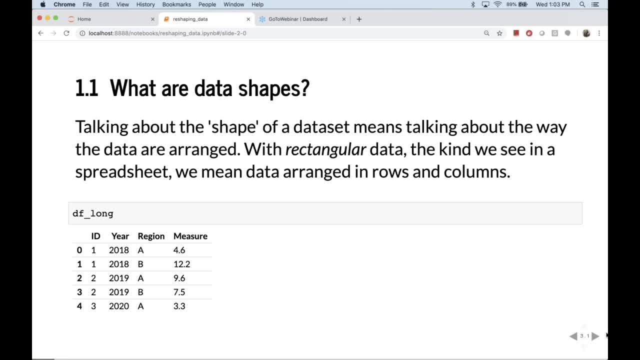 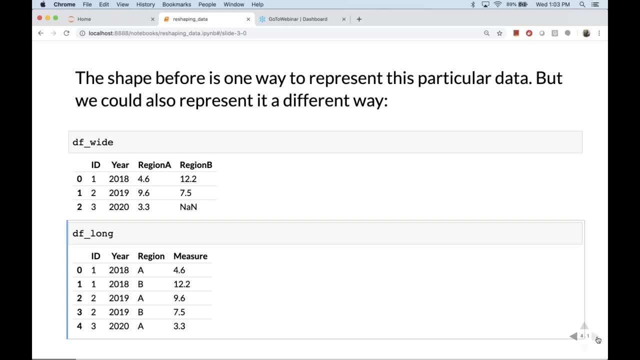 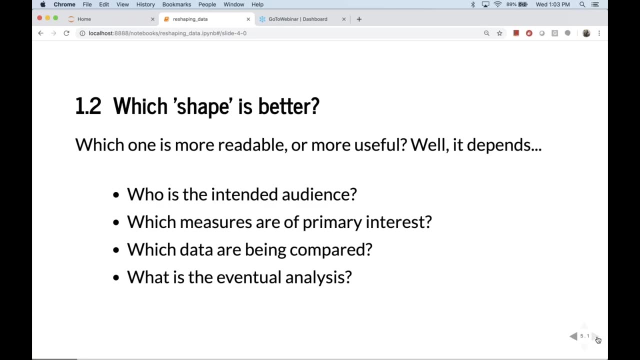 4.6, 12.2, exactly, and then the data rearranged into this other shape, Right, and we can see that there. So which shape is better of these two shapes? Well, it really depends on the context. Which one is more readable or more useful to you. 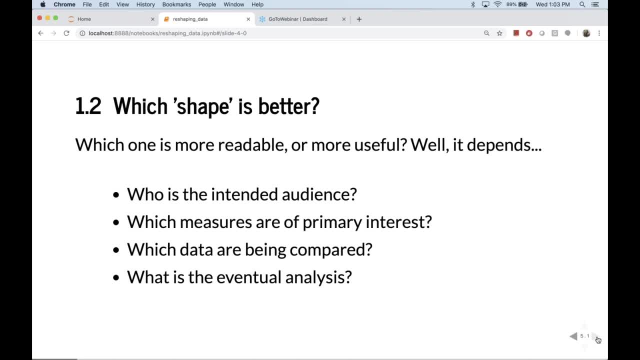 Depends who your intended audience is. Who are you trying to talk about this data with? Who are you trying to show it to? Which measures or variables are of primary interest? Those are the ones that you want to focus on and make sure that you want to ensure are clearly displayed. 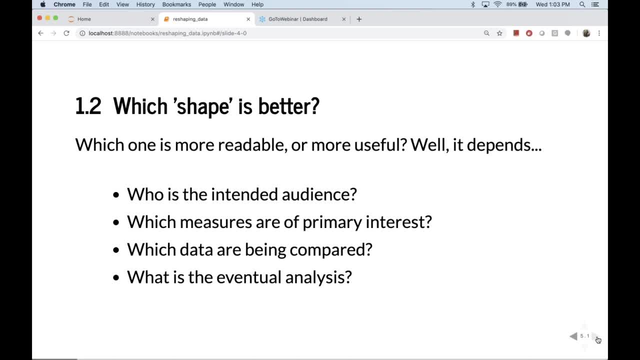 Which data are being compared. In the previous wide format maybe we were looking at the differences between region A and region B and we really wanted to highlight that And that second format, that wide format, would have been more clear in that regard. 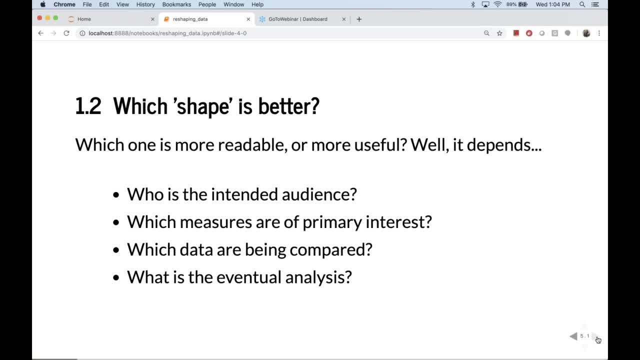 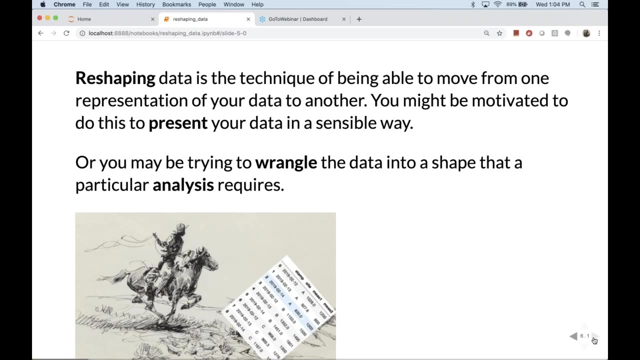 Or another goal that you may have is: what is the eventual analysis? What do you want to do with this data That may drive the shape that you try to arrange this data into? So, reshaping data generally is this technique of being able to move from one representation of your data to another. 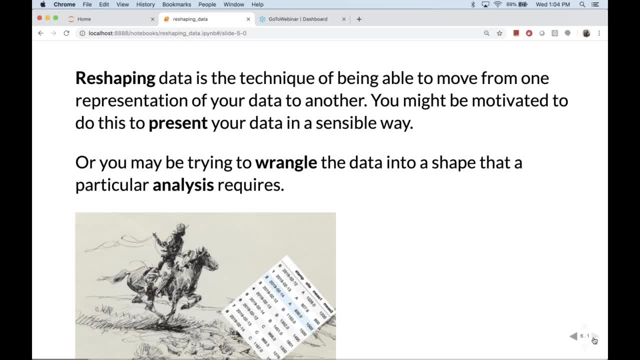 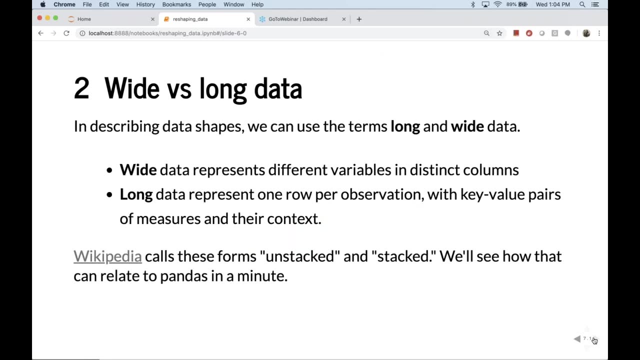 You might be trying to wrangle the data- there's another verb for it- into a shape that a particular analysis requires, like a visualization or model. I'm going to zoom out here a little bit on my slide. So again, some basic vocabulary here: wide versus long data and describing data shapes. 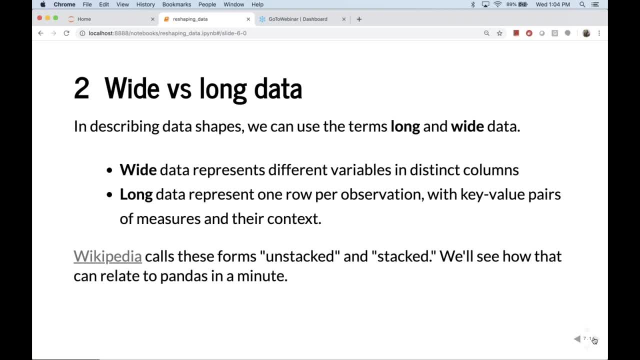 we can use the terms long and wide, Wide data and there's different definitions of this. this is just one definition. Wide data represents different variables in distinct columns and it's a very natural way of arranging data, especially when we think about adding data to a spreadsheet. 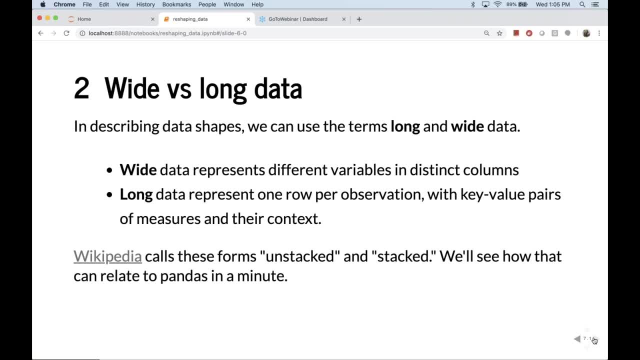 Long data, on the other hand, represent one row per observation, often with key value pairs of measures in their context. So another variant of this. on the Wikipedia definition, if you look up long and wide data, you'll see that they also call these forms unstacked and stacked, and that's going to. 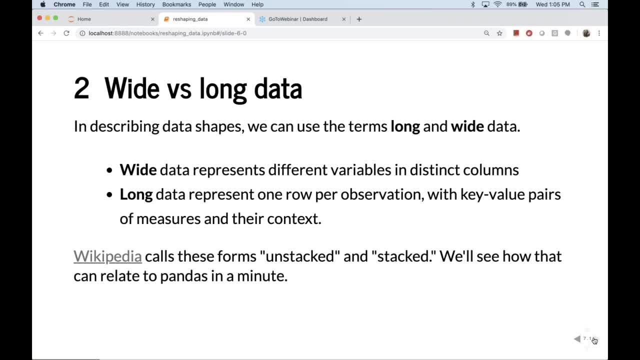 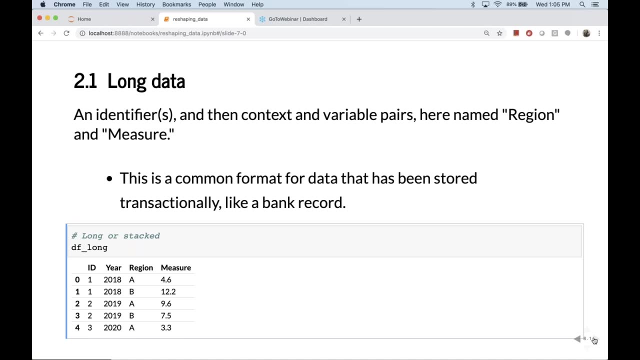 track nicely to some of the Pandas methods that we have available to us. We'll see that as we get into Pandas here in just a moment. So again, what is long data? Long data is usually this transactional format of data when we have some kind of ID variable. 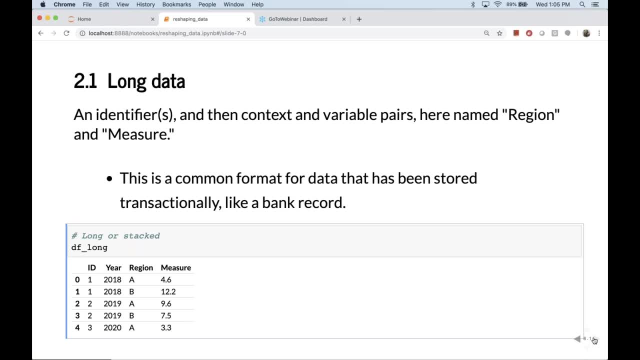 or ID variables that describe unique observations. Sometimes it can be one or more variables as a combination that create this observation identifier, And then we have context and variable pairs. In other words, in the example that we have below, we have these measures per region. 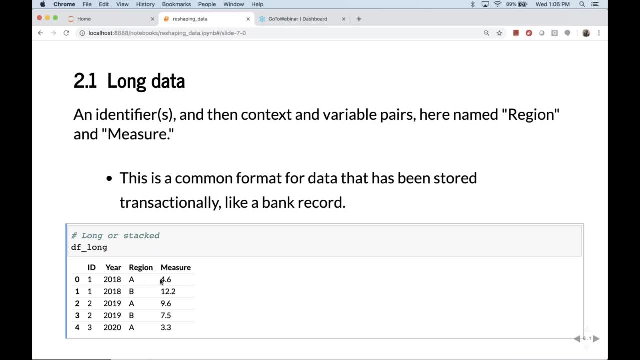 and then we have a separate column that describes which region these measures belong to. Is it region A or region B? right, And we can think of the ID and year columns together as being those unique identifiers per observation, And this is a common format for data that's been acquired or been stored transactionally. 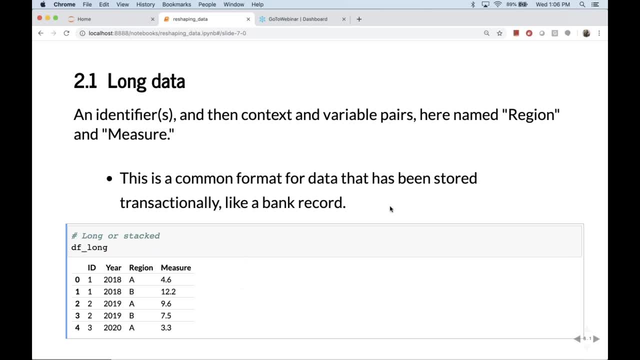 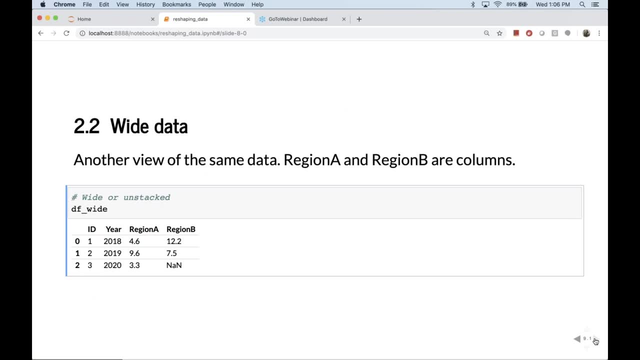 like a bank record Or some kind of ledger. Another common way of describing data is wide data. This is the same data that we had before, but region A and region B are distinct columns now, And this is a useful display of data because we can compare for ID number one in the year. 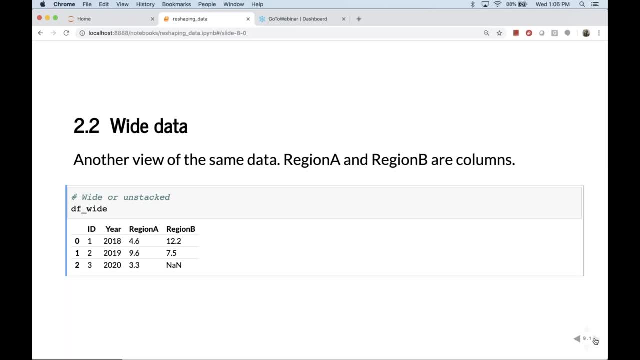 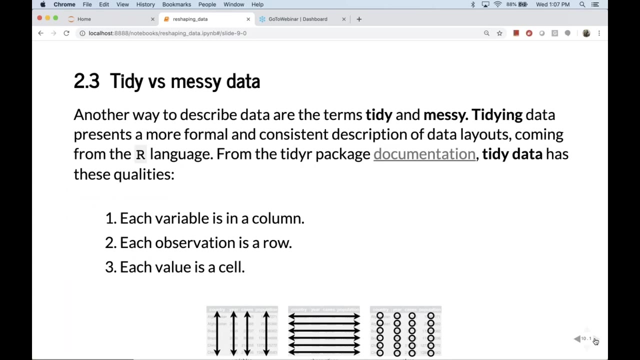 2018 how region A and region B differ from each other. So it was one of these data. Is one of the shapes better than the other? Is one more correct? Not really. It really depends on what your usage of this data is going to be. 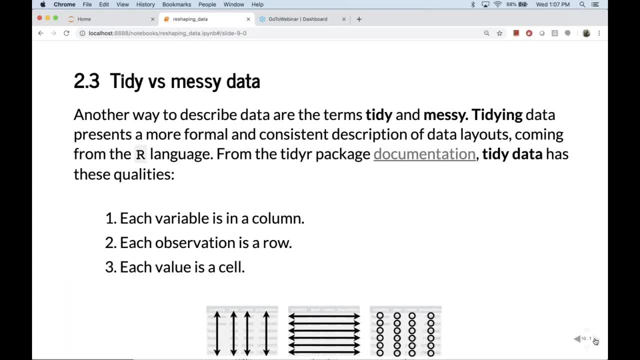 There is another way of describing data and this is coming from the R language and the R world. There's a popular methodology in R which is a statistics language, computer language, And those terms are tidy and messy. You might have heard of these if you've heard of something in the R package library called 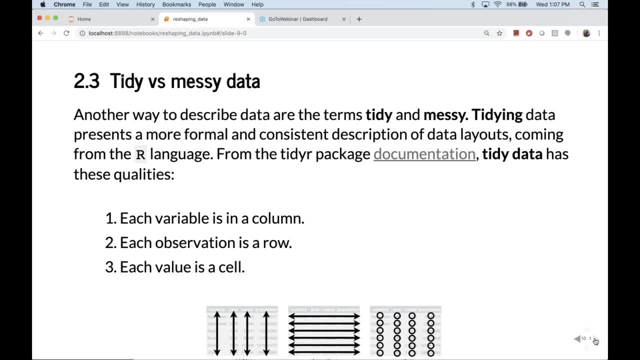 the tidyverse, And this is a more formal and consistent description of how data can be laid out So tidy. data in this definition has these qualities: Each variable is in its own column, Each observation is its own row And each value is a cell. 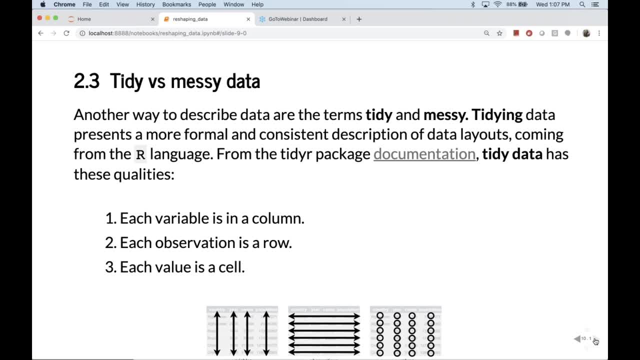 And you can see a little graphic of that here at the bottom of the page. So again, each variable is in a column. So whatever our variables of interest are, they're going to be in their own distinct columns. Each observation is a row. 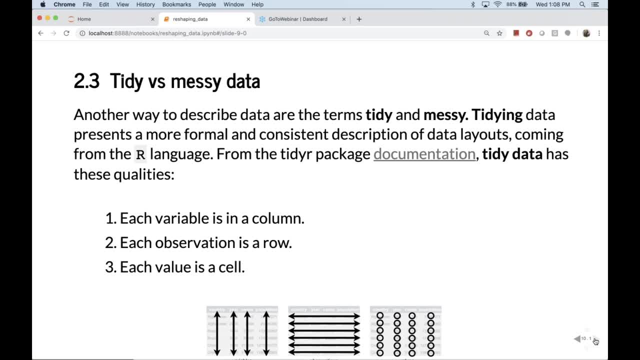 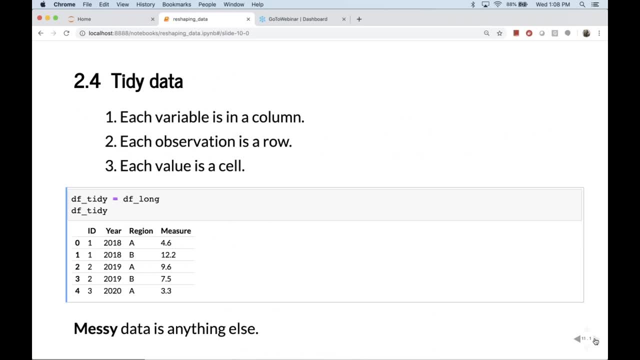 And then the values fill in the cells. So that's a definition. We can use that as a working definition of tidy data. So in our context, these little data frames that we've had as examples here, what does tidy data look like? 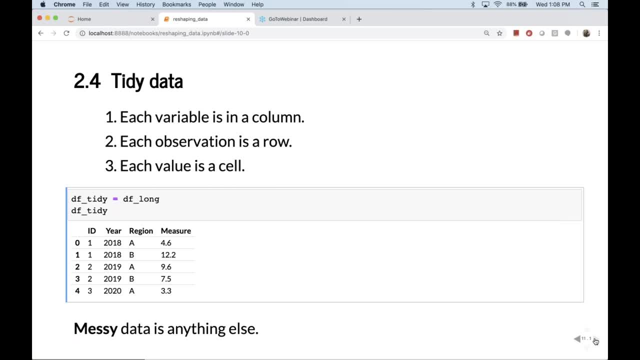 Well, this could be a version of tidy data here, What we had as the line. It's a long data format, but it doesn't always correspond to that exactly. But here we have each variable in a column, So we have a column for region. 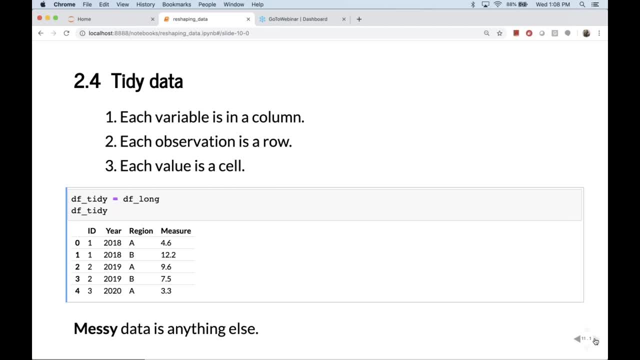 And then we have a column for the measure. whatever that measure is, Each value is in a cell. So we have, for the years 2018 or 2019, region A or B, and then the values of the measures, And each observation is a row. 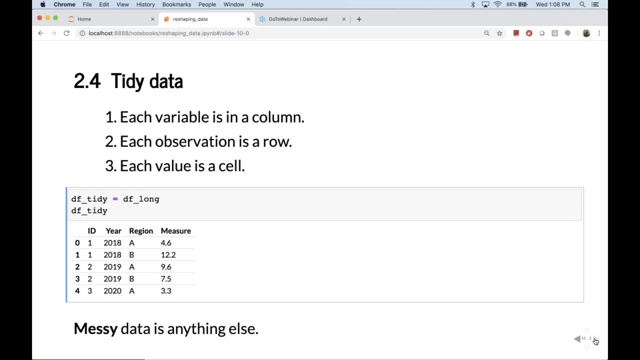 So this could be considered tidy or tidy-ish data, And the contrast to that is that it's a row. It's a row, It's a row, And the contrast to that is messy data. Messy data would be anything else that doesn't fulfill these principles. 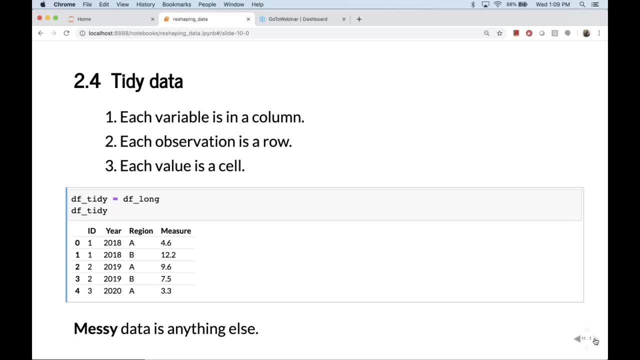 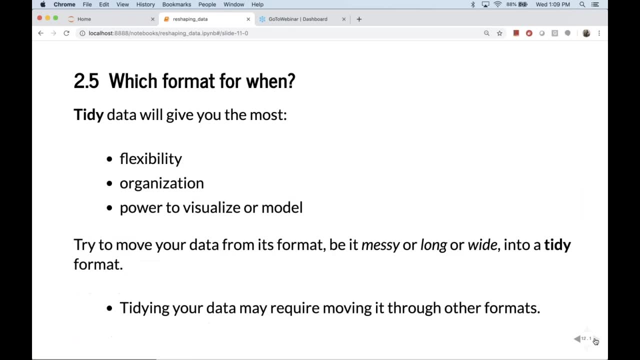 Now, this is not hard and fast rules. Again, it's just a framework for thinking about how to arrange your data. So, which format do you need and when do you need it? Well, in general, if you work towards making your data tidy, tidy data will give you the 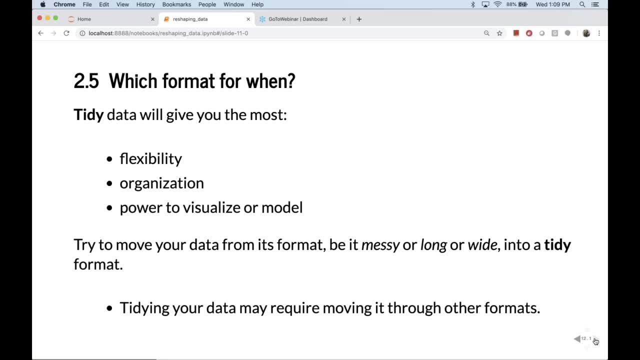 most flexibility, It'll give you the best organization and it'll give you the most power to take further steps to visualize or model your data. So if you get some data in and you're not quite sure what to do with it, maybe your 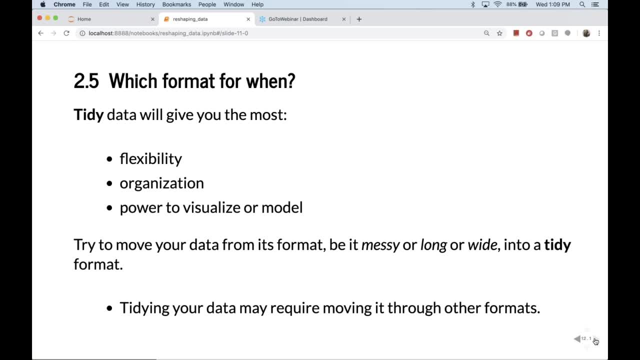 first step should be to think about how you can tidy it, So to move it from whatever format it may be coming to you in, be it messy or long or wide, into this kind of tidy format that fulfills these principles And that process of tidying your data is very important. 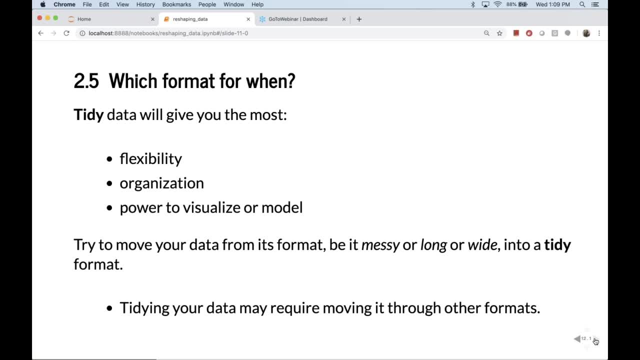 It's very important. It's very important, And the data may require moving it through other formats, be they long or wide, or taking subsets of your data. And these are just general guidelines. Again, this is just one way to work, to think forward if you're not sure what to do with. 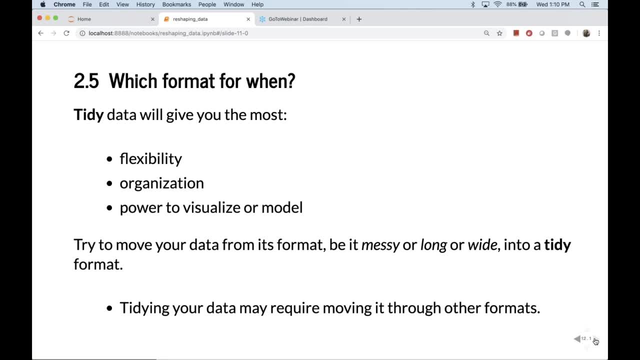 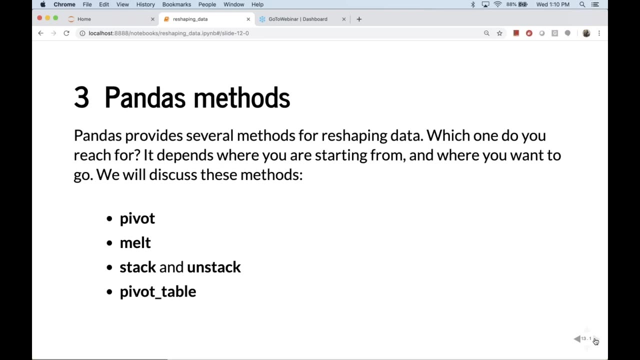 your data, And we'll show you some resources at the end of the webinar on some tutorials online that take several different cases of data and move it through messy formats into what they consider a tidy format. How do we accomplish this In Python? Well, with pandas, we have several methods for reshaping data. 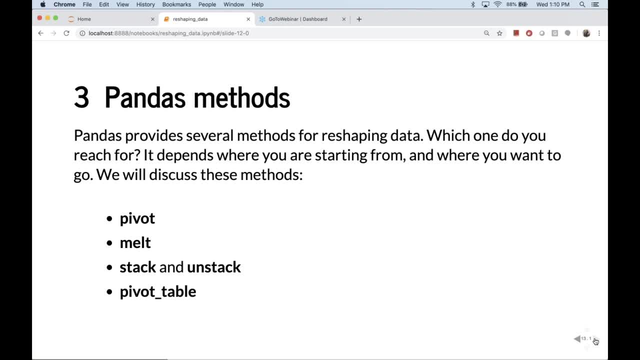 Which one do we reach for? Well, again, that's going to depend on where we're starting from, what format our data is in and where we want to take it. We're going to talk about these methods in the pandas library. the pivot method, the. 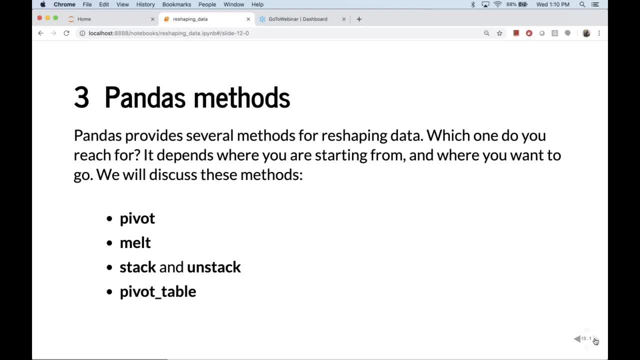 melt method, the stack and unstack methods and the pivot table methods. Now there's other methods, There's other functions in pandas that you could consider to be part of the reshaping world. Things like transposing your data or even doing things like group buys could also be. 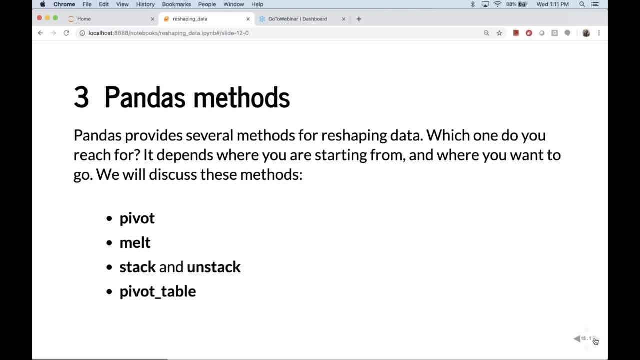 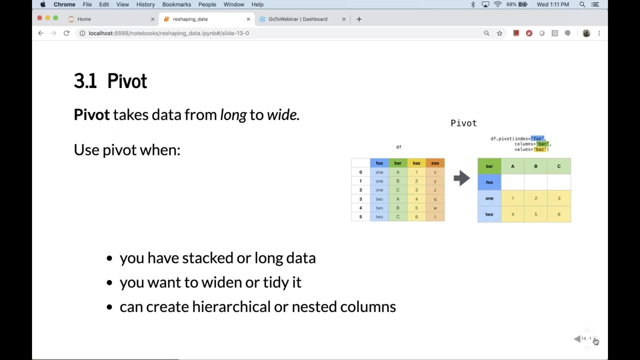 considered reshaping your data. We'll take a glance at some of those, but we'll really focus on these five methods and look at the differences and similarities between them. So we'll start here with pivot, And if you're familiar with the vocabulary from spreadsheet programs, you're probably 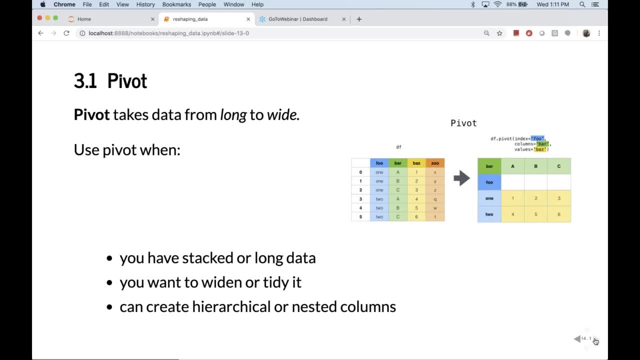 familiar with the word pivot And if you're familiar with the vocabulary from spreadsheet programs, you're probably familiar with the word pivot. You might have heard of a pivot. You might sort of know what a pivot is. This is the way pandas is going to think about the pivot and this is what its pivot method. 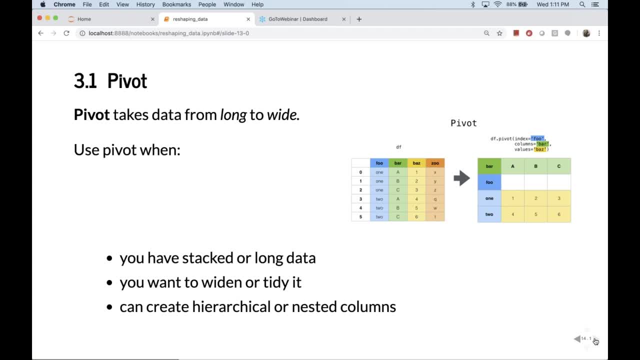 specifically means Pivot is for taking data from long to a wide format, And these graphics that you see on the slide here, the multicolored data frames, are taken directly from the pandas documentation. So if you go to the documentation, you'll also get a lot more information, more details. 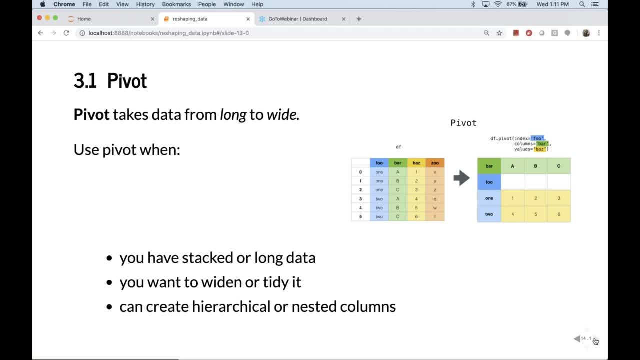 on these methods as well, Beyond what we're showing you here. So pivot will again take this data from long to wide. So you have stacked or long data. You want to widen them or tidy it, And pivoting can create hierarchical or nested columns. 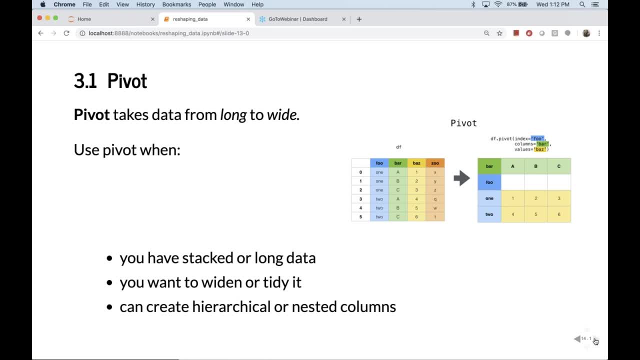 So when you do that- move from this long or stacked data, depending on how you pivot, you might get hierarchical or multi-indexed columns in the results, And we'll see an example of that in a minute. So pivot is for taking data from long to wide. 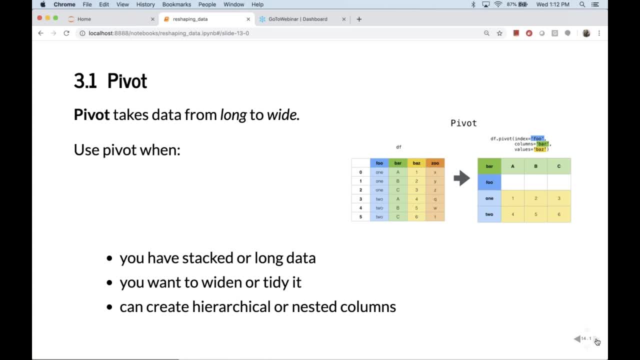 So you have stacked or long data. I'll show you an example of that in just a moment. So in this graphic, what we're seeing here is that this data has been pivoted from this long format using the index foo. The new columns are the. 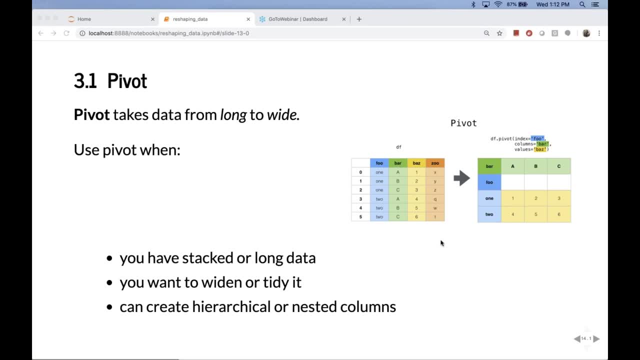 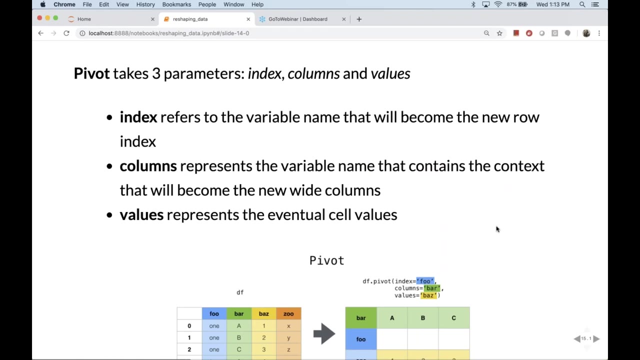 green column bar. we've dropped the zoo column and the only values that we're using are the yellow column, as Am interested by Pivot's data Text on screen. Pivot takes three core parameters: index, columns and values. Index refers to the variable name that will become the new row index, the new row indices. 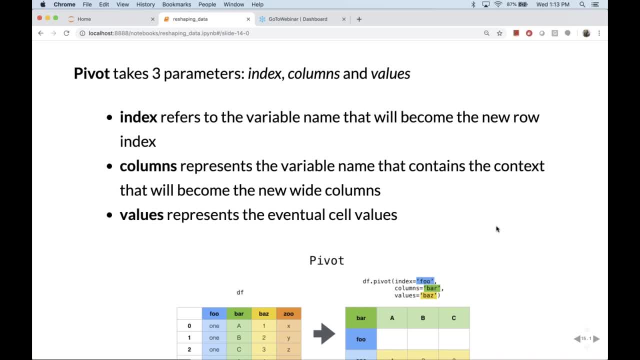 Columns represents the variable name that will contain the context that will become the new wide columns. So, whatever it is that you now want to spread horizontally across your rectangle, that's what the columns values are going to be. And finally, values will represent what goes into those cells. 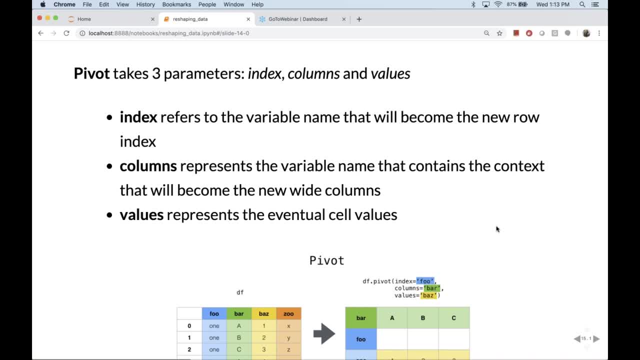 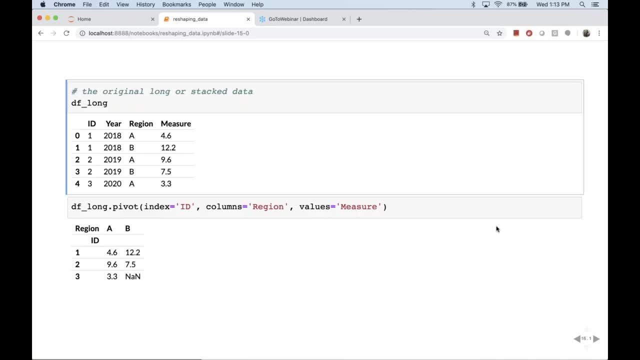 where are those numbers or values being taken from? So here's our original long or stacked data. Again, we have the ID column, we have the year column, we have a region column and we have a measure column. And if we pivot this, 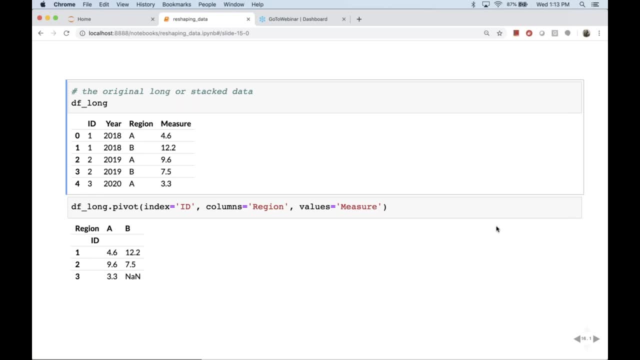 on the ID column with our region column as the new horizontal column index, spreading it out across the regions with our values coming from the original measure column we get data frame below So we can see that we have our IDs are now the data frame index one, two and three. 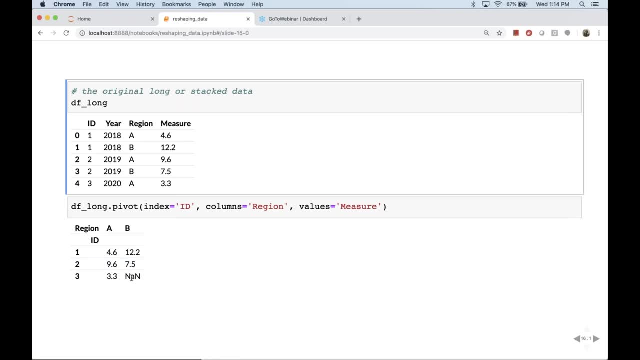 We have two columns, A and B, and the measures are populated inside of those. Now there's something a little funny here. There's this region on the left-hand side. We'll look at that and see where that came from in just a moment. 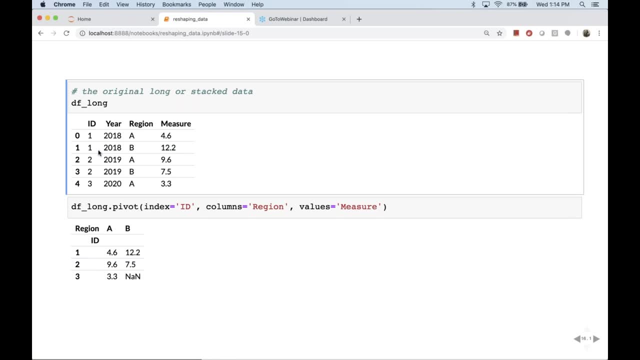 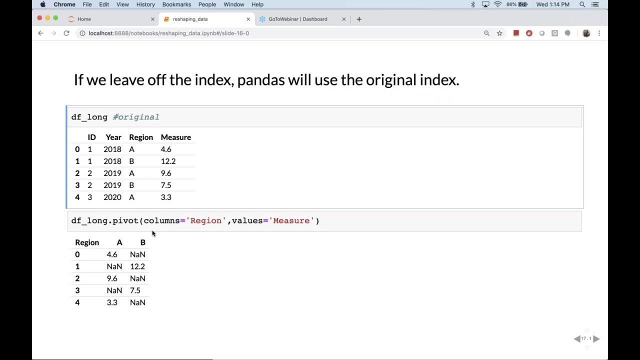 So this pivot again has taken the data from this long format to this wide format. We don't have to supply an index with this method. We can just leave off that index parameter. If we do that, then Pandas will try to use the original index. 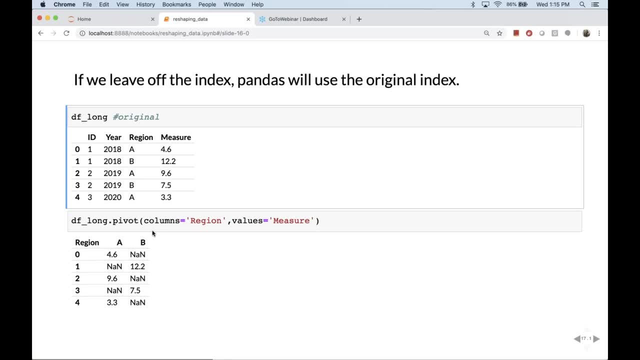 In this particular case, if we do that without the index, it'll still create those A and B columns here, but it'll fill in missing values where it doesn't have values for row zero, the original row one, two, three and four. 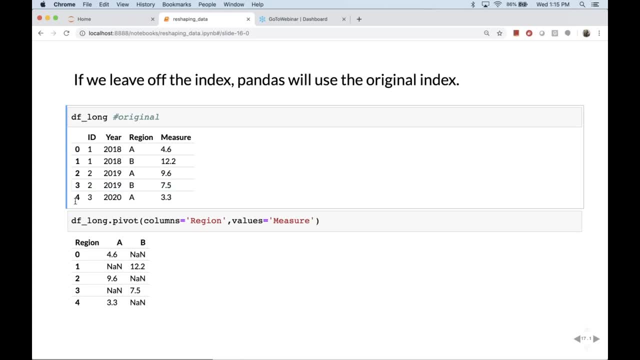 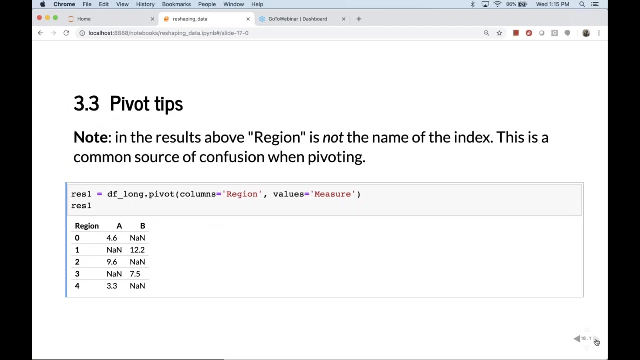 So you can see, it's borrowing that index from the original data frame index. The data frame long here and it's dropped that ID information again because we've only given it this: columns equals region and values equals measure. So notice that when we did that result. 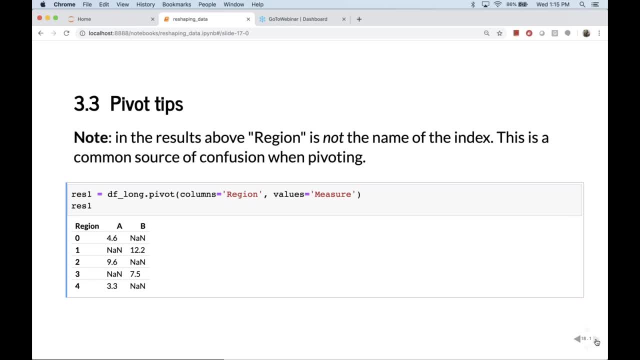 we got this region showing up at the top level there- boldface. I'm using a Jupyter Notebooks here in slide mode. That's what you're seeing in terms of the display here And that can be a source of confusion when you're pivoting. 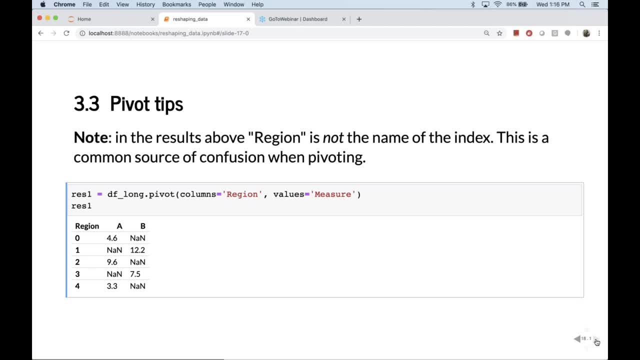 Sometimes people look at that. You may sail right over it, It may not be a big deal to you, but sometimes, if you're showing the data to other people, they're looking at that and they're saying, hey, what is region zero and region four? 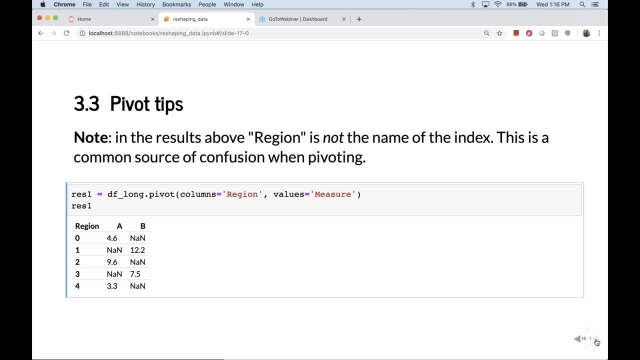 I didn't think we had these regions, And it's just a little bit of a display issue here And that it looks like region is the name of the index column, which it is not. So how do you get rid of that? Well, what you can do is just look at the columns attribute. 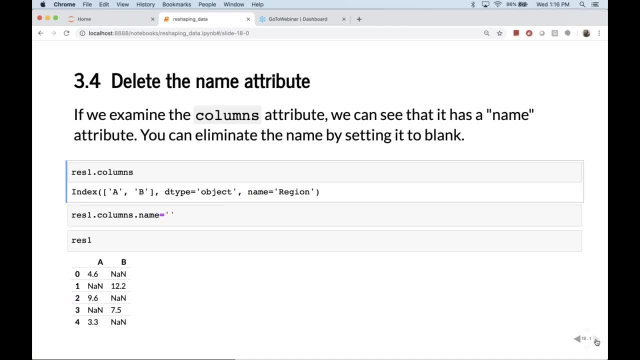 of your resulting data frame. So in this case we've named the resulting data frame res1.. If we look at its columns attribute, we see that it has a name attribute. name equals region. We can just set that to an empty string. 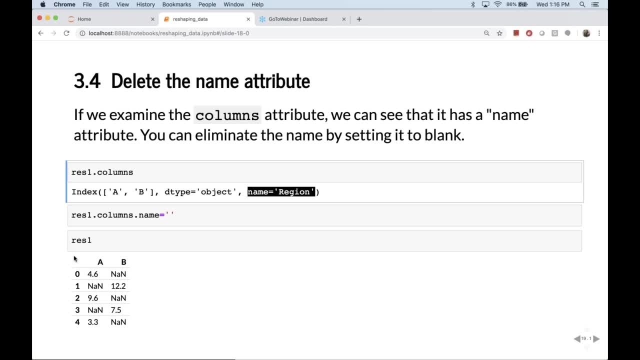 and then we get rid of that region. So if you have a column attribute, you can just set that to a new header in the display And again this can just be a little source of confusion. You can be wondering where it comes from. 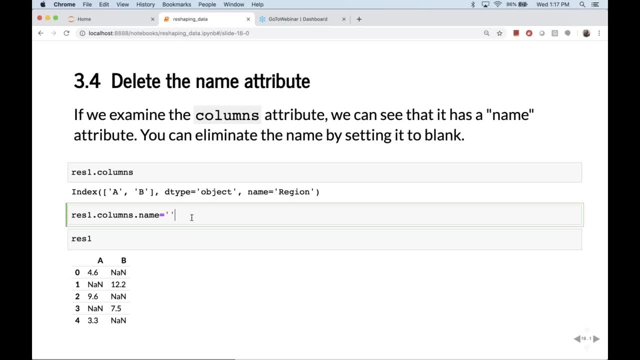 especially when you pivot into multi-columned, multi-indexed columns. Sometimes that can look a little bit strange there And if you just look at the columns attribute of your results you can eliminate that retitle it whatever you want to do with it there. 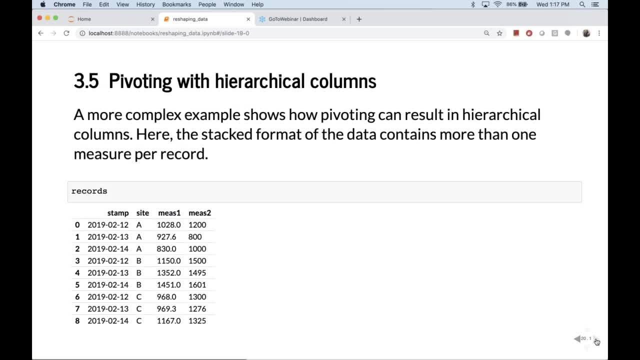 Here's another example data frame And we're going to show how pivoting here again, taking from long to wide, can result in hierarchical columns in the output, In other words, a multi-column index in the output. Here this stacked format: 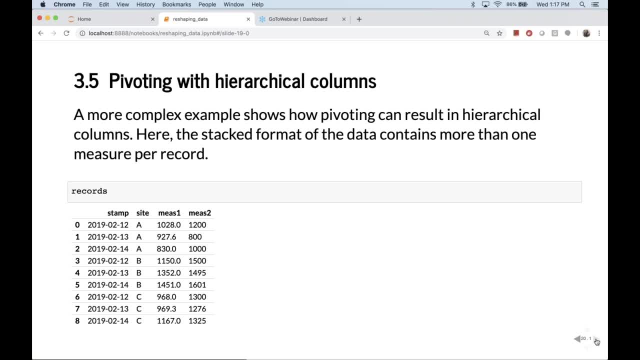 this long format of the data contains more than one measure per record right. So we've got these timestamps, February 12th through the 14th, and sites A, B and C, But for each of those we have two measures. 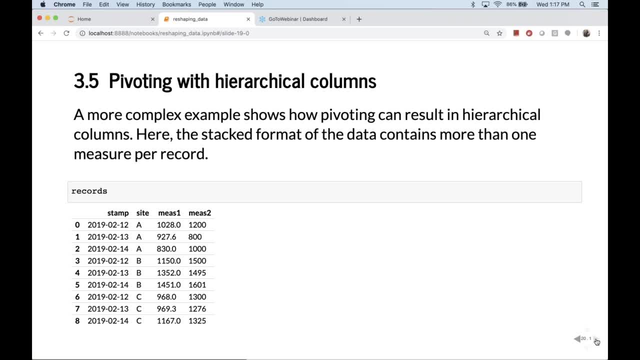 measure one and measure two. So again could be another example of some kind of transactional data that we have here. If we pivot this, if we take it from this long format to wide, let's say that we want to spread it across the horizontal- 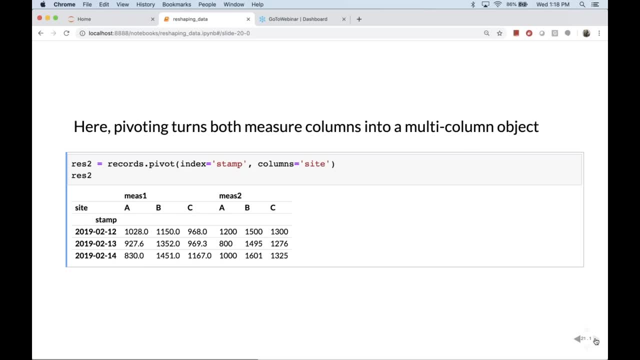 for display purposes, for easier reading here. We're going to keep that time index as the row indices there. So index equals stamp. Our columns are going to be the site. but you see, in that result what we have are two subsets of data. 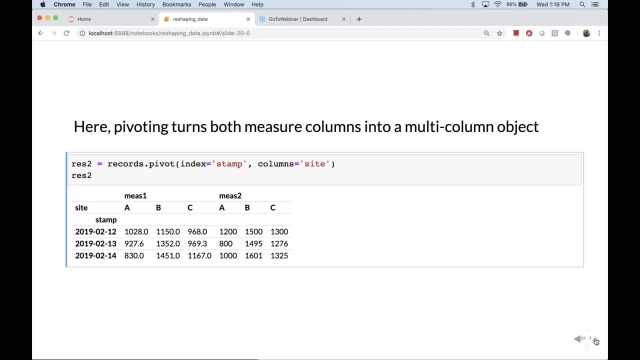 So we have site A, B and C per measure one and measure two. In other words, we have this hierarchical multi-column index here, right, We've got two levels of the column headers. We've got measure one and measure two. 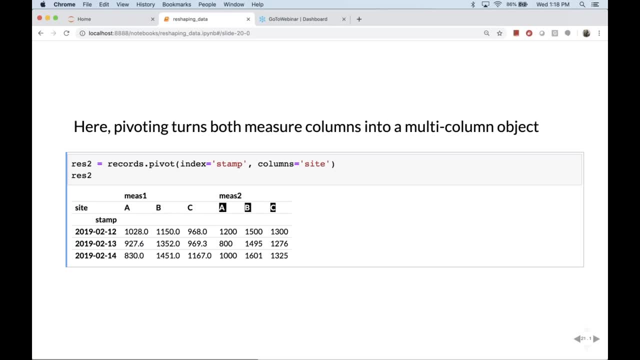 and then sites below that- A, B and C, and A, B and C repeated. So this can be a result of a pivot. That may be something that you want, and multi-indexed data can be very useful. So if you have multi-indexed data like this, 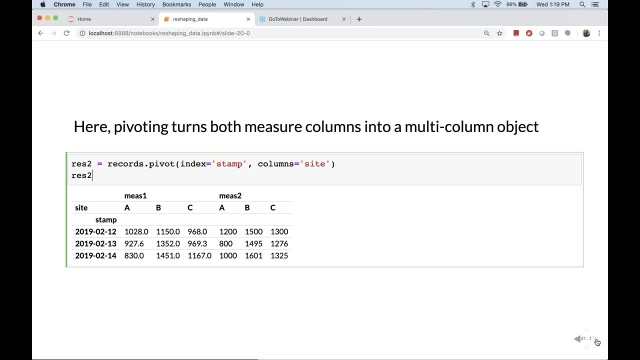 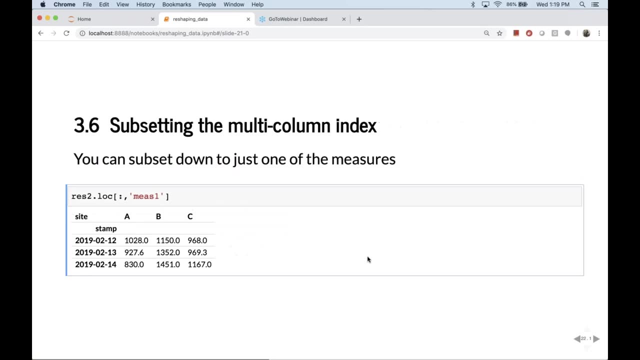 in this case, multi-column data. you can subset it down. Pandas gives you lots of nice ways to subselect data in these kinds of formats, So if you wanted to select it down just to measure one, you could do that with a loc. 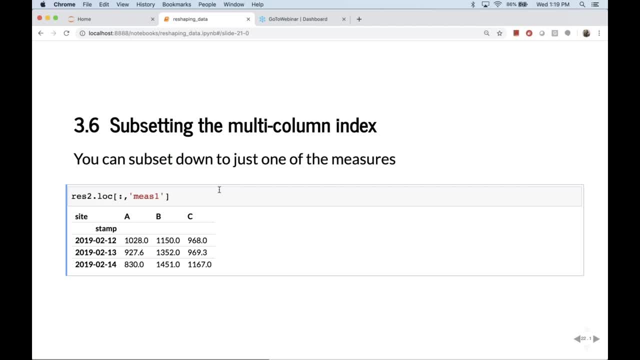 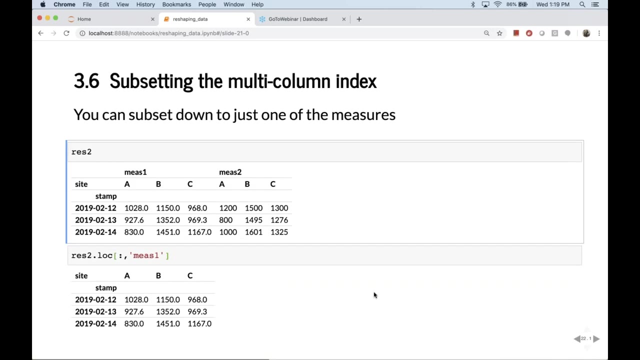 So here we're using loc to pull out sites A, B and C, but just from measure one So we can see the. I add the original results and then you can see the subset there below right. So this is one way that you can subset that data. 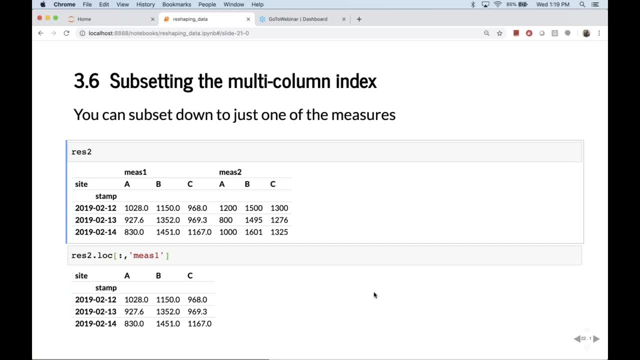 after you've done the pivot, Something that a multi-column index will allow you to do. What if we wanted just the A columns out of this resulting data frame? How would we get that? We could use something called index slice to get and again loc. 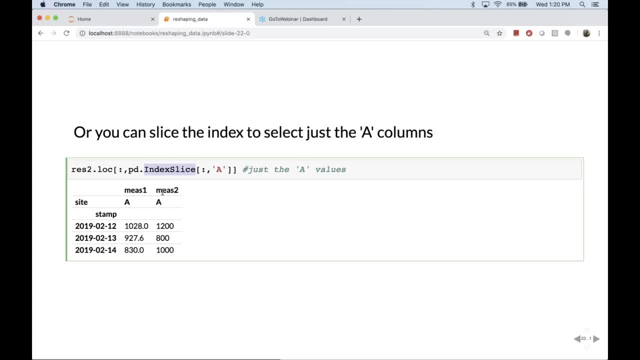 but we could use the index slice method to get from measure A and measure two, from measure one and measure two, just the A columns. So that's how you could possibly deal with multi-column indexing. So that's how you could possibly deal with multi-column indexing. 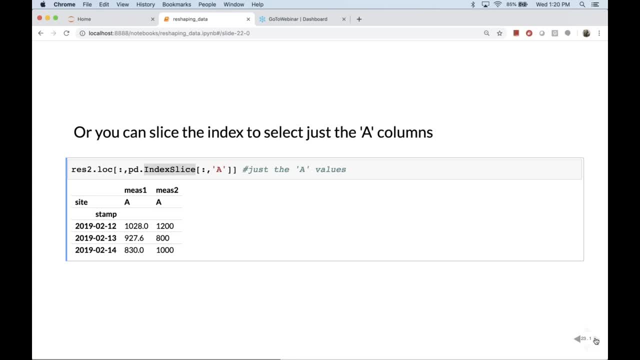 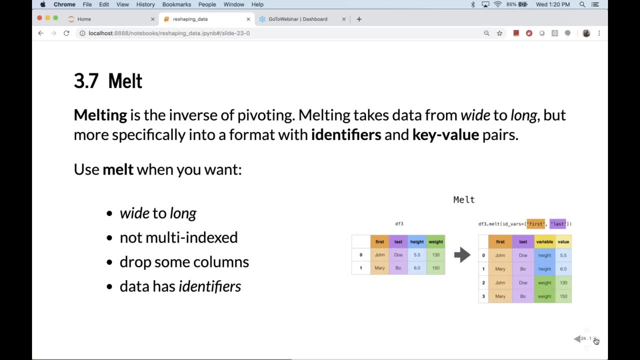 as a result of a pivot. So again, pivoting takes your data from long to wide. The inverse operation of that is something called melting. Melting takes data from wide to long, but more specifically, it takes it into a format with identifiers. 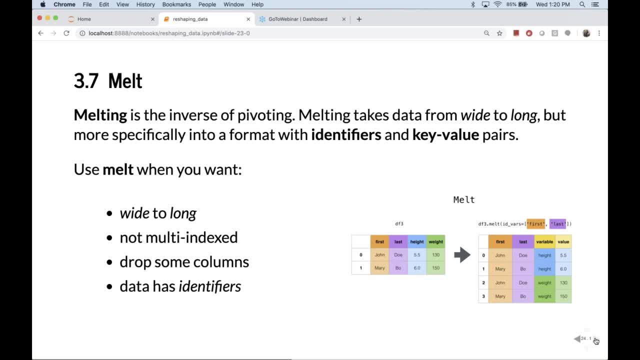 and key value pairs, or context value pairs sometimes they're called. So you're going to use melt if you have data that's coming in a wide format and you want to turn it into that transactional format. The data isn't multi-indexed. 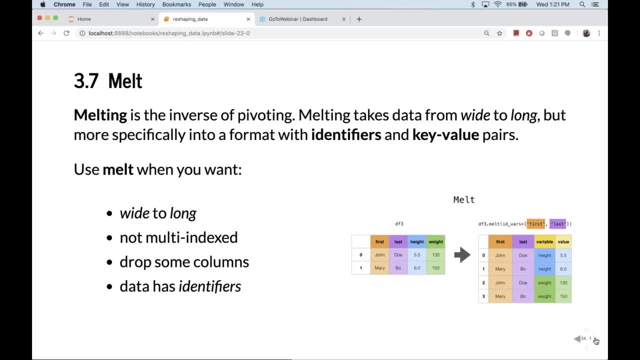 it's just simply indexed. Maybe you want to drop some columns in those results And when you're doing this your data will probably have an identifier or identifiers, maybe a column or more than one column that will make up that unique identifier per row, per observation. 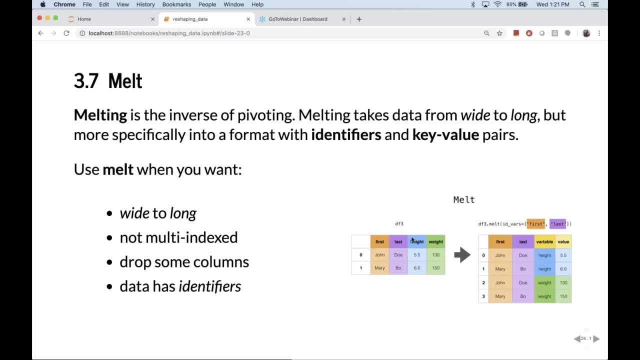 So here's a little graphic, again taken from the Pandas documentation of melt. We can see that first and last the orange and purple columns are the identifiers for the records, And we're taking the blue and green columns height and weight. 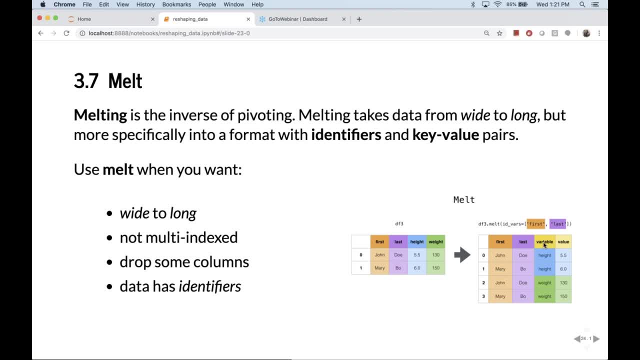 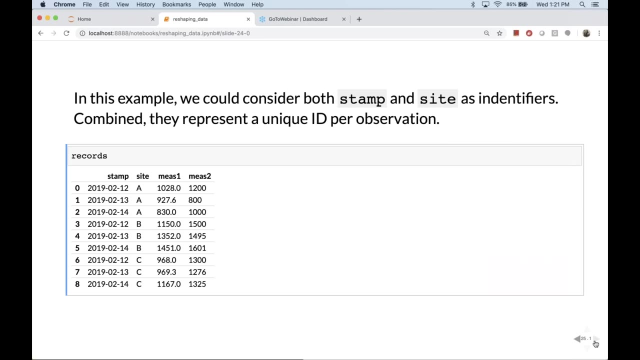 and turning it into these yellow columns of key value pairs or variable context and value pairs. Let's look at another example of that. Here's our records data set again with our timestamps and our sites, And maybe we want to take measure one and measure two. 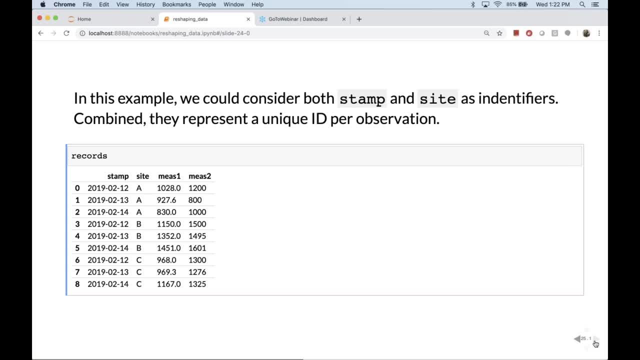 and turn this into. we said that this was a long format or long-ish format before. maybe we want to turn it into a strictly long format now. So we're going to use length So we could combine stamp and site and together consider those unique IDs per observation. 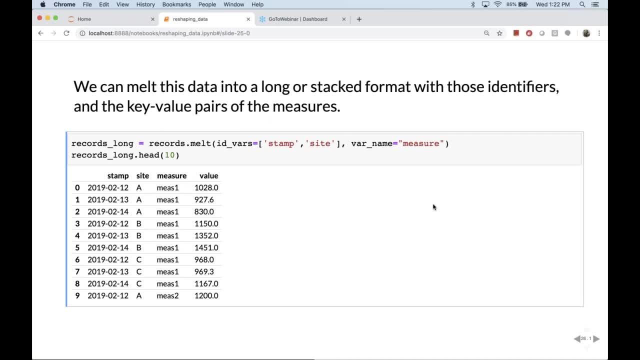 So here we're looking at just 10 of the results We're selecting. we're using our ID VARS parameter to select stamp and site columns from the original data frame. We're going to use our ID VARS parameter to select our ID VARS parameter. 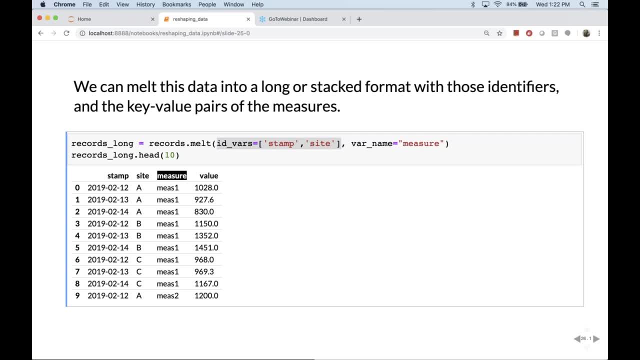 and we're going to rename this column here: measure. We could have left it the default, which had just been a variable, as you saw in the previous example, but here we're renaming it to measure. So now we have a strictly long data set. 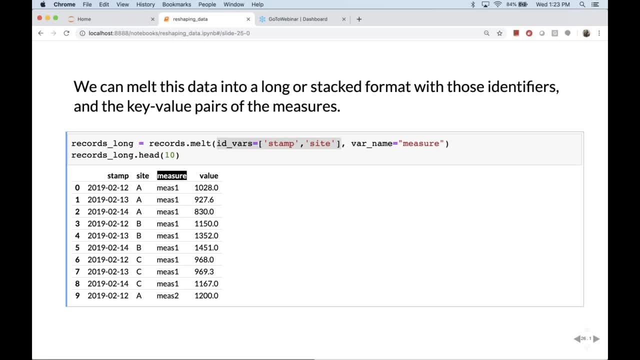 We've truncated it to 10 records here, but, as you can see, what it's done is created a record for measure one and its value. measure date: February 13th. site: A measure one and its value, And then we'll repeat those records. 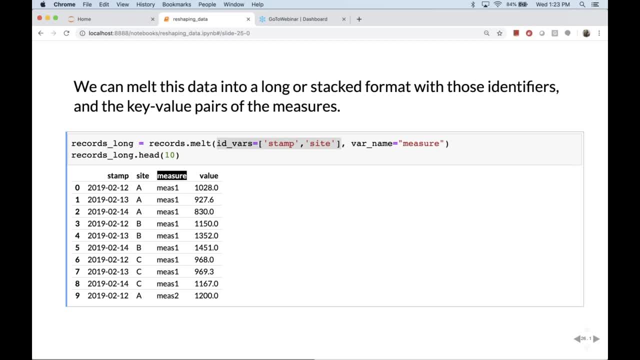 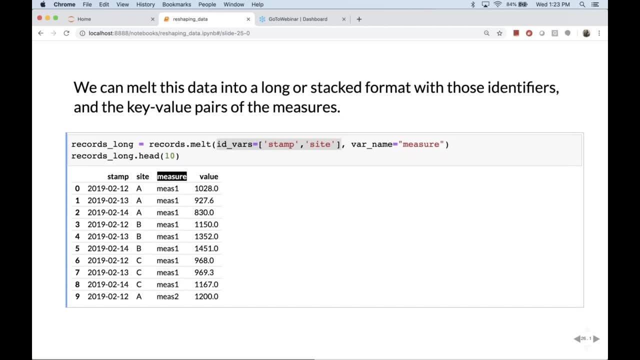 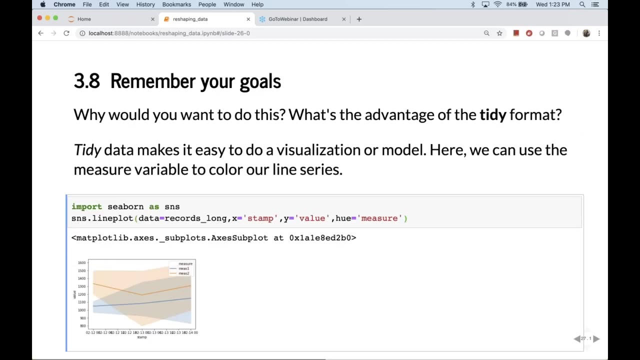 for the same dates and same sites for measure two. So it's taken- what was that previous data? and turned it into a strictly long format here. Why would you want to do this? What's the advantage of a tidy or a long format like this? 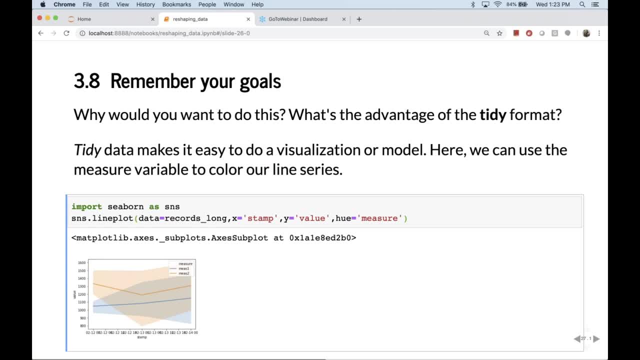 One reason that you might want to do it is because you want to visualize or model your data Here in this format of records long, and we've melted it in that way. we can use the measure variable to color our line series. So here we're using a Seaborn plot, just a line plot. 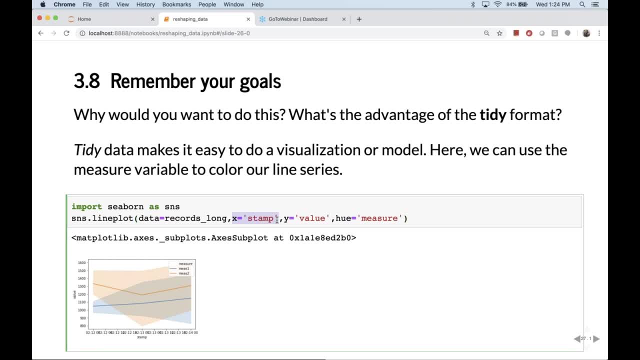 We're taking our X axis from the stamp parameter and I realize this graphic is pretty small here, but it should give you a little bit of idea of why we're doing it. in this case, Our values are going to be the line values. 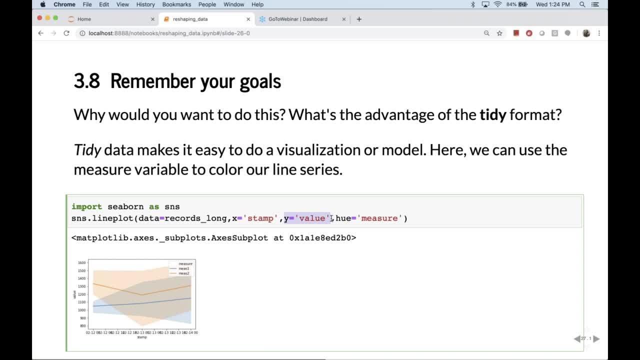 So we'll make the line series here and we're able to easily color those two line series based on that new measure column. So this is one way that you could do it. You can also do line series with the Y data, but this is a common format. 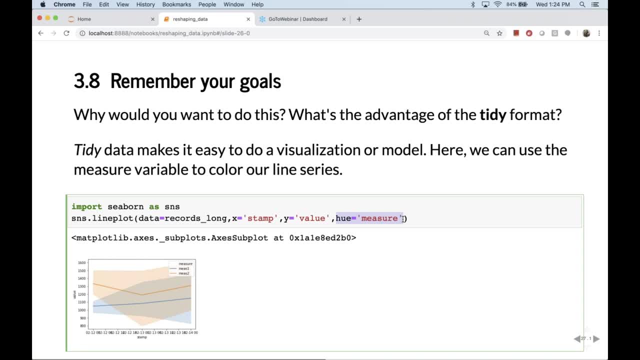 if you want to color your data by a particular variable or set the size or line type and the visualization by a particular variable. So that's one reason. visualization routines often like your data in a long or strictly long format, So that might be one reason. 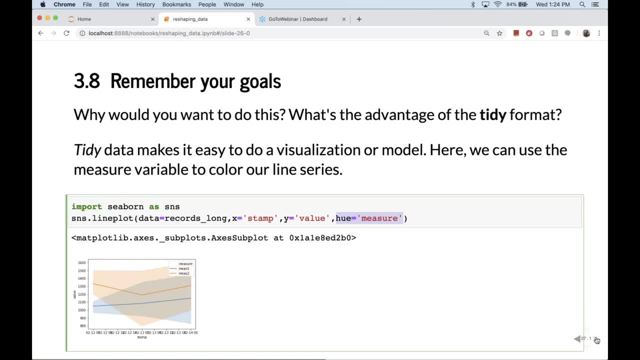 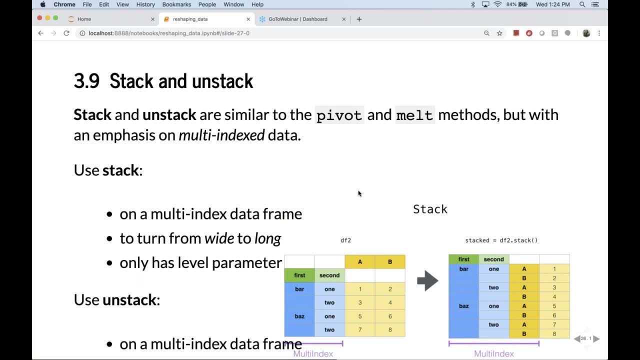 that you need to reshape it in this way. So that's pivot and melt, which are the workhorses of reshaping your data, but there are other methods available in Pandas to do this And some of those that you might have come across. 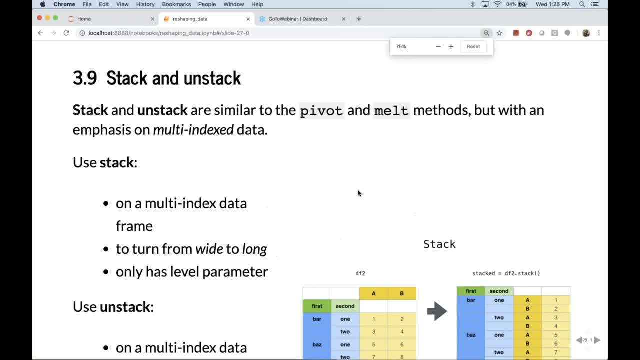 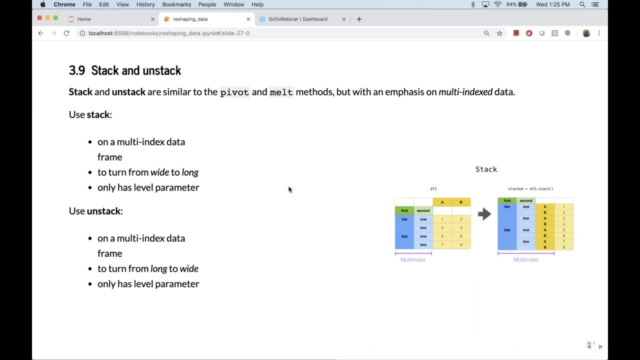 are stack and unstack. I'm going to zoom out here on the slide just a little bit so we can fit all this information on. So stack and unstack are similar to the pivot and melt methods, but they have a more specific usage. 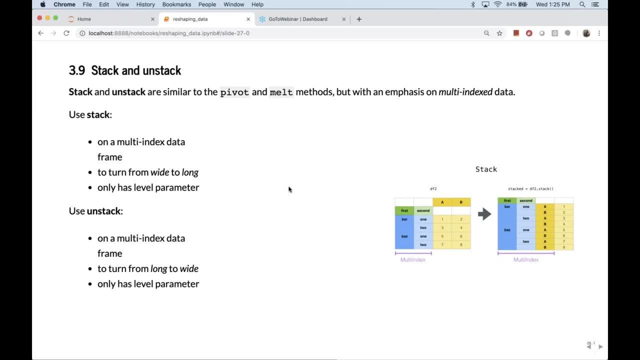 and they don't have quite as many parameters available. Stack and unstack expect multi-indexed data, So they expect that what you're putting into these methods have some kind of multi-column index or multi-row index. Stack is going to be a little bit different. 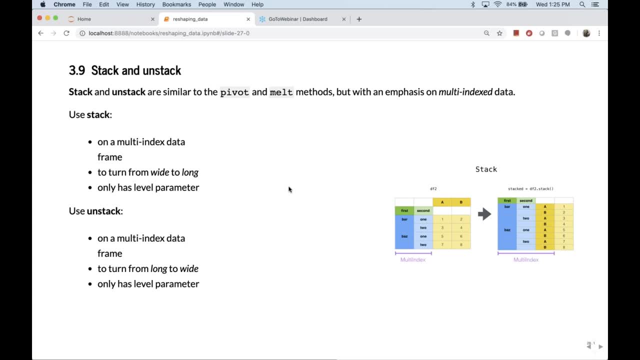 It's going to be the method that you want to use. if you have that multi-indexed data and you want to turn it from wide to long, It only really takes one parameter, which is the level parameter. There's a drop in A in there as well. 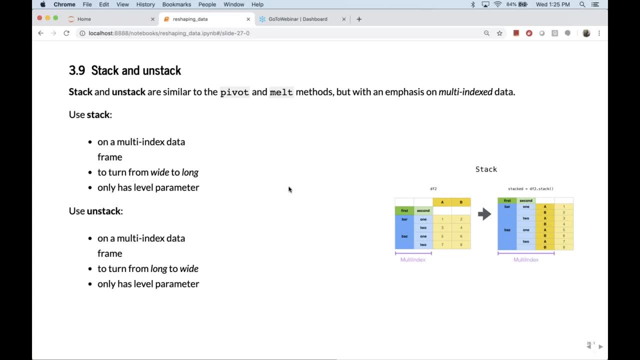 but we'll just concentrate on the level parameter. Unstack similarly expects a multi-indexed data frame. It's going to turn it from long to wide and it also only really takes a level parameter, and we'll see some examples of what that means. 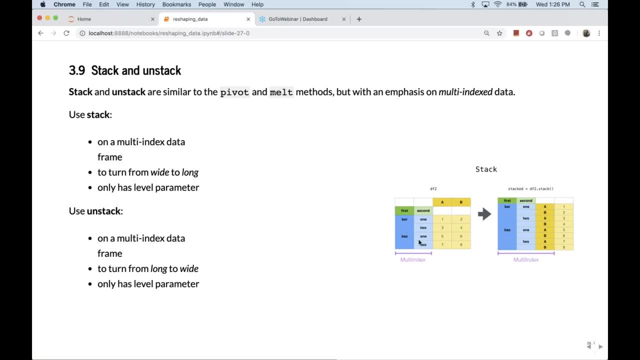 So here's a wide data set here with a multi-index. We've got these first and second columns as our index and we're stacking it or we're turning it into long, and we now have a three-layer multi-index and the results with first, second. 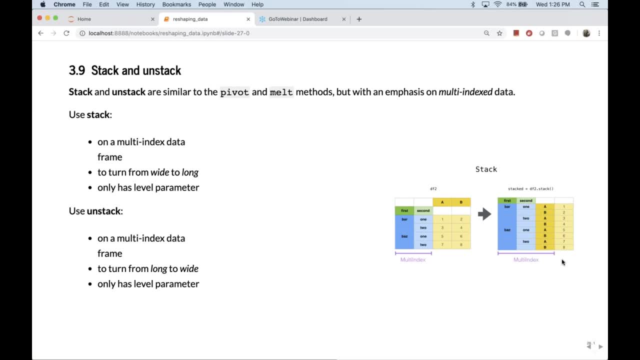 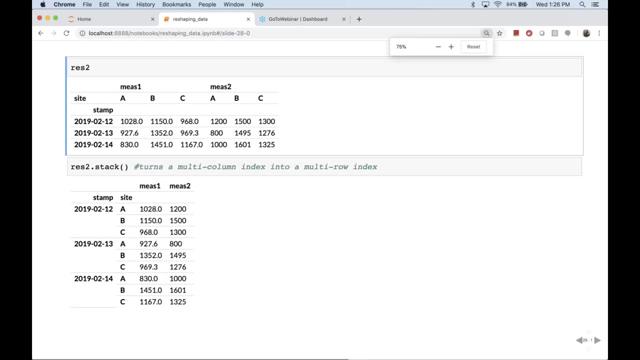 and then A, B, A, B, going down the rows and our values in the last column there in the example that you see. So with our data, let me zoom back in here so it's not quite so tiny. Here's our multi-column indexed res2,. 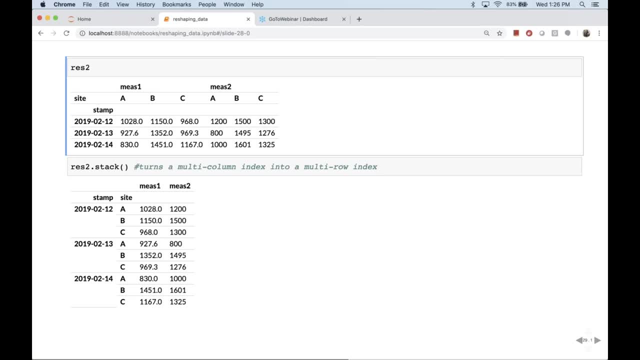 our wide data that we made with our pivot method and we can take this and we can use stack to turn it back into a long format. So you can see it's taken that level of the site and turned it into a multi-indexed object there. 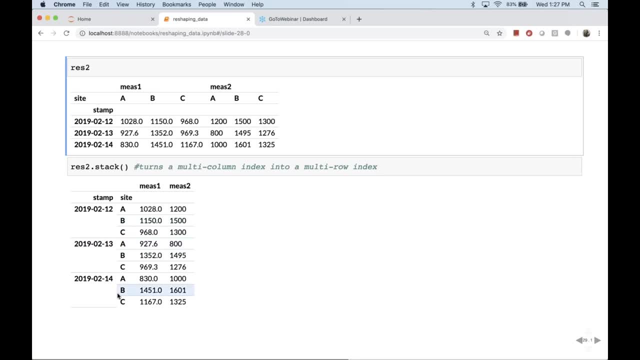 So we have stamp and we have site. Now in this display that we've created, we have stamp and site on the left-hand side as a multi-index for this new data, the results of this res2 stack. Sometimes what you want to do, 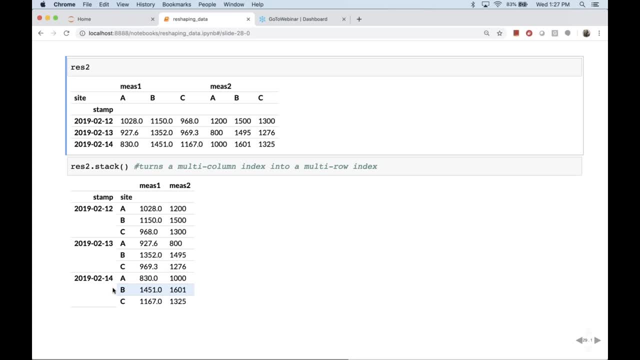 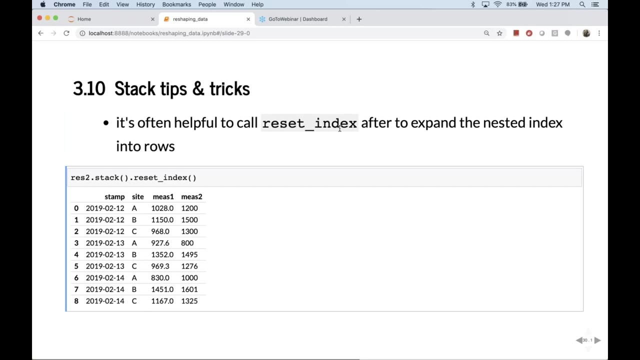 after you make this move is you want to expand these indexes, these multi-indexes, into true columns, and you can do that easily with the reset index method. So this reset index method is often useful after you do something like a stack, to expand those columns out into true columns here. 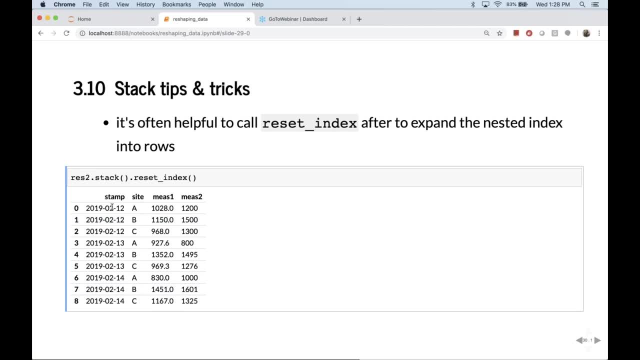 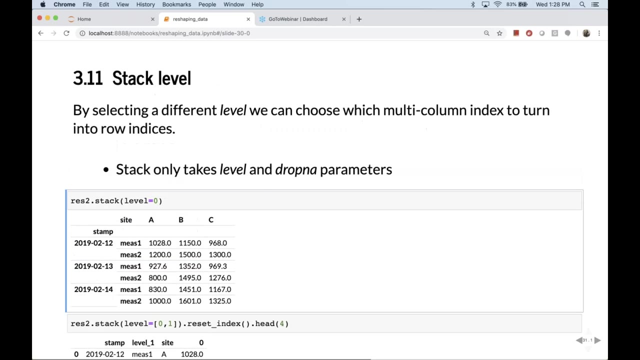 So you can see that you have a new column stamp with the values to February 12th through 14th And site ABC. So again, reset index is often helpful after we call stack, By changing the level here we can again. that's that one parameter. 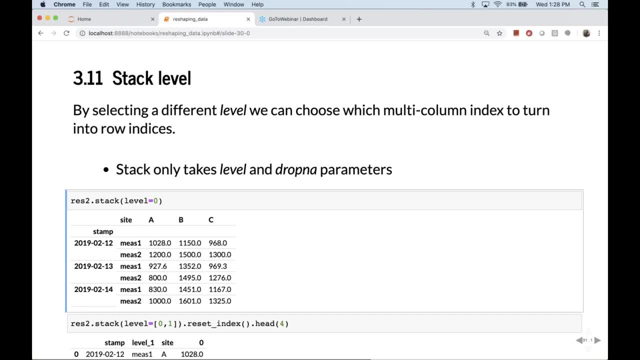 that stack and unstack will take or the main parameter that they'll take. We can choose which index of the multi-column index we want to turn into the row indices. So by default it shows that site level, but we can adjust that if we want to. 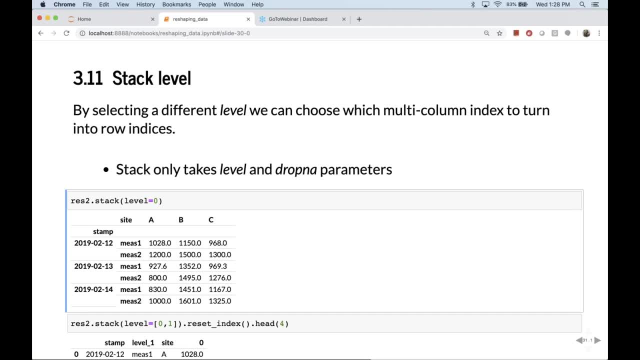 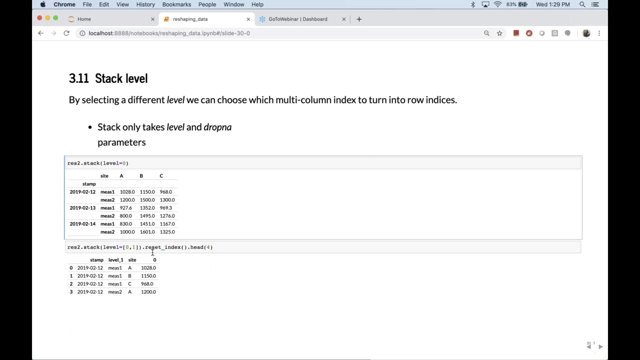 So here, if we say stack level equals zero, instead of stacking on the site index it stacks on the measure index. So you can see measure one and measure two in the results. Let me zoom out a little bit more here So we can see. 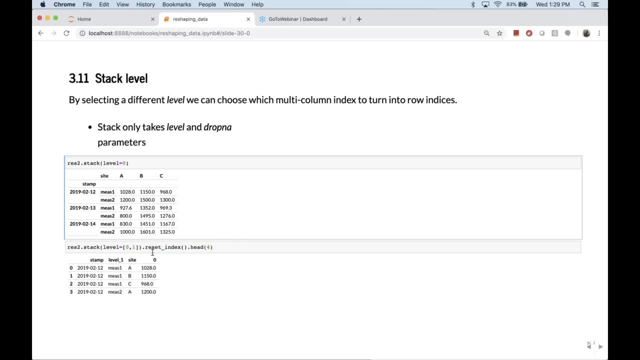 we can also pass it a list or list-like object to that level parameter And we can ask it to stack on both the measure and the site and get that truly long format which may be what we want there. So you can see that here. 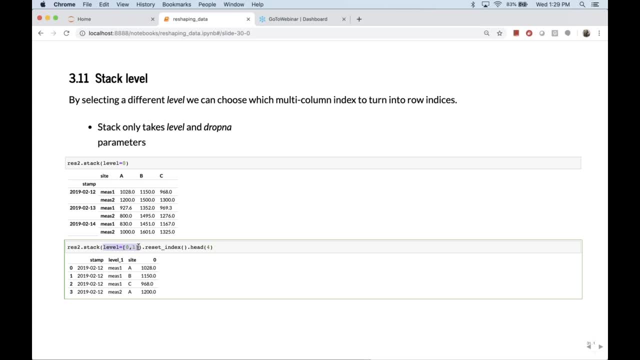 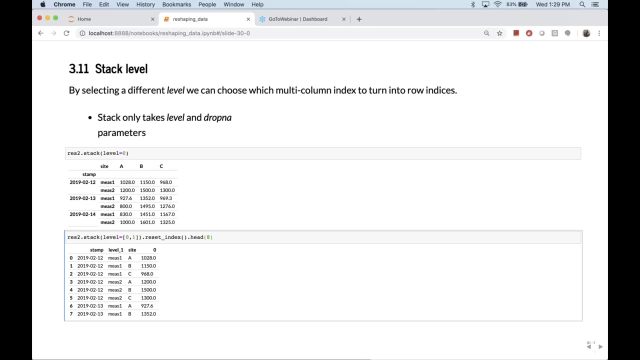 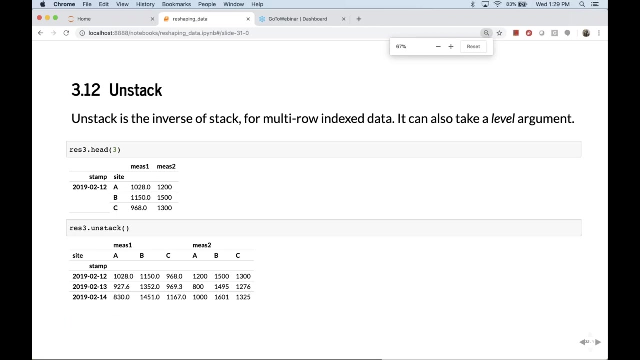 we've passed the level parameter- both levels zero and one- and then reset the index. You've chained the method onto there. Excuse me, You can see what the results look like there. Similarly, unstack is the inverse of stack for multi-row indexed data. 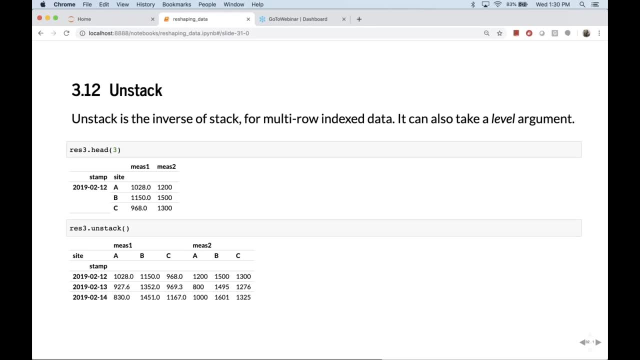 Also takes a level argument. So we're going to use unstack when we have a multi-row indexed and we want to turn that into Y data. So we're doing a lot of just shuttling our data back and forth to show how these methods complement one another, right. 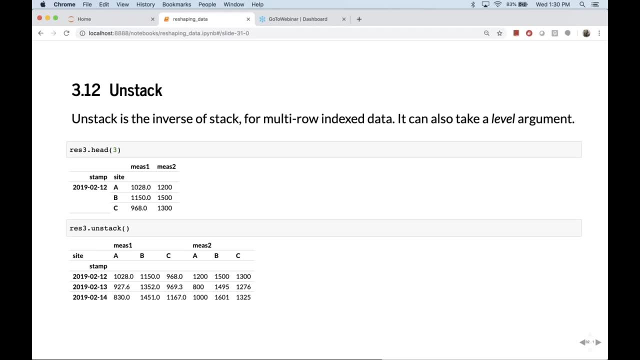 So one is the inverse of the other. So here we have res3 again. This is just that. I think we'll get a few more rows of it. This is just that: multi-indexed, multi-row index data. That was a result of a previous operation. 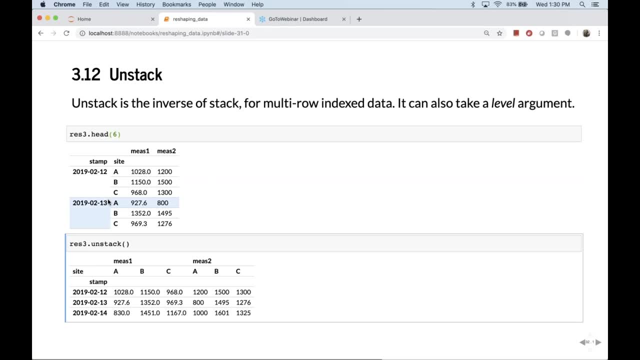 So that's the result of a previous operation There. What if we want to widen, that? We want to turn site on the horizontal as columns across? We can do that in this case with unstack. So stamp remains. This outer index remains as the index here. 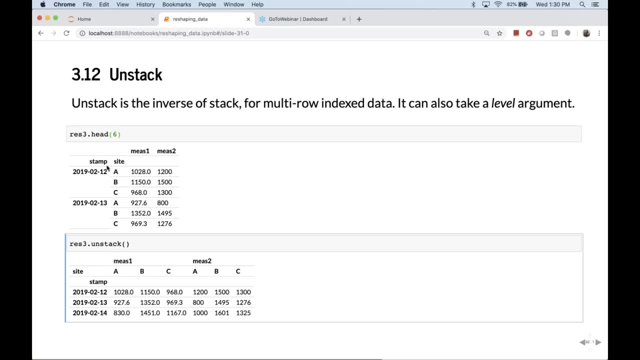 But now we have a multi-column index, again with measure and site. So this is from long or longish format to a wide format here with unstack, And again we can choose which level we want to unstack. So if we wanted to put the dates across, 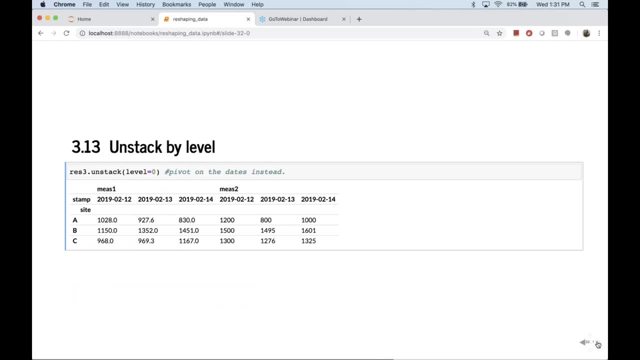 instead of the sites. we could do that by changing the level, And, of course, you can play with this and play with different levels to see what your different results are. So again, we've got four methods here, but they expect slightly different incoming data. 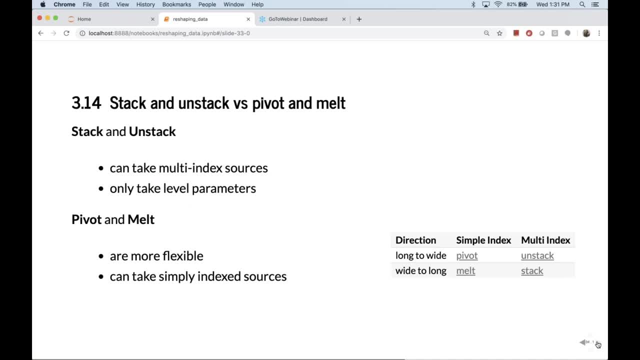 and give you slightly different results and have a little bit more time to think about how we're going to use them, So you can use the same method to look at different results and have different parameters. Stack and unstack are for when you have multi-index sources. 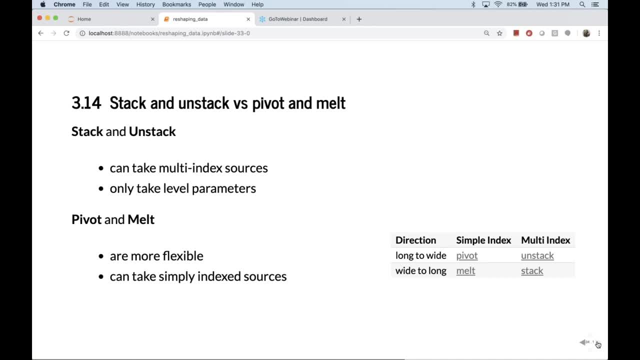 They only really take level parameters. so they expect those multi-index and they're just for turning from long to wide or wide to long. And here's a little table of what those do. Pivot and melt are more full-featured. They're going to take more simply indexed sources. 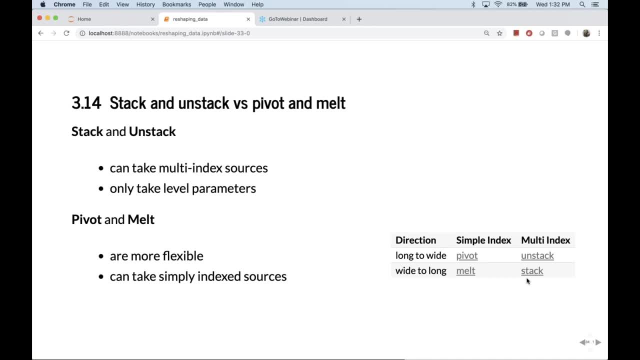 but they could make multi-index data as an output. but they're going to provide you more flexibility. They're going to ask you: what do you want to keep as your ID? variables? Which values, which measures do you want to spread out or gather? 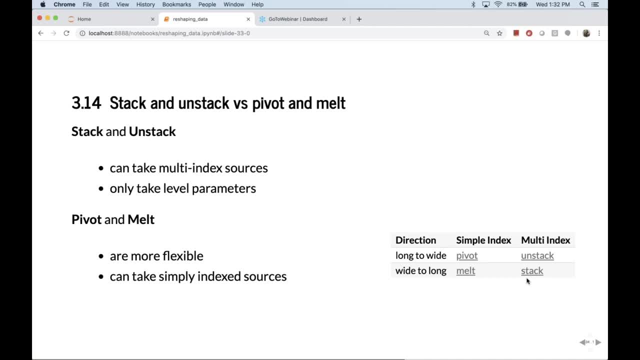 So your main methods are going to be pivot and melt, But again, that depends on your incoming data. here, If you already have multi-indexed data sources, you might be using stack or unstack. So what about this other method that you've probably looked into? 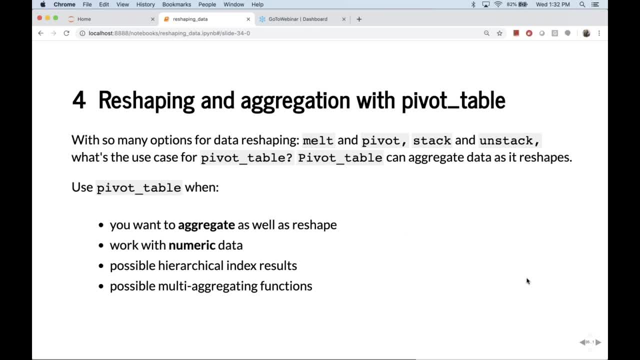 or run across, which is pivot table. You've got so many options for data reshaping, melt and pivot, stack and unstack. When do you use pivot table? Well, pivot table is a little bit different. It is that idea of reshaping. 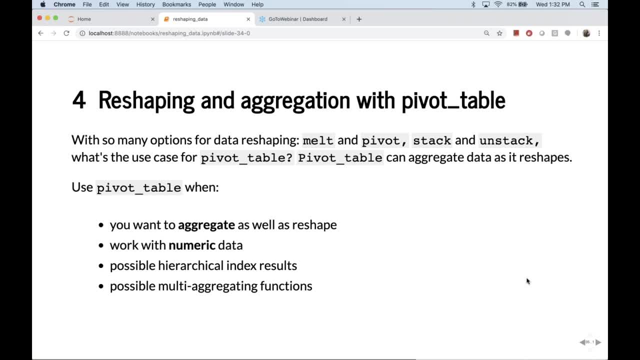 but it also does aggregation. So when you want to change the shape of your data but you also want to accomplish some kind of aggregation- whether it is calculating a count or a sum on the number of records- that's when you're going to reach for pivot table. 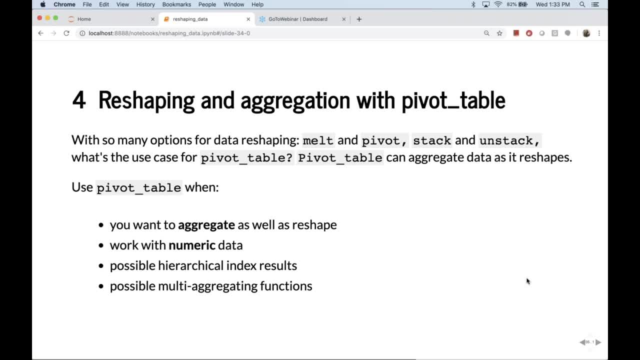 It works with numeric data, So the measures are going to be numeric as an output, It can possibly create hierarchically indexed results, And it's also possible to use more than one aggregating function, And we'll see some examples of that here in just a minute. 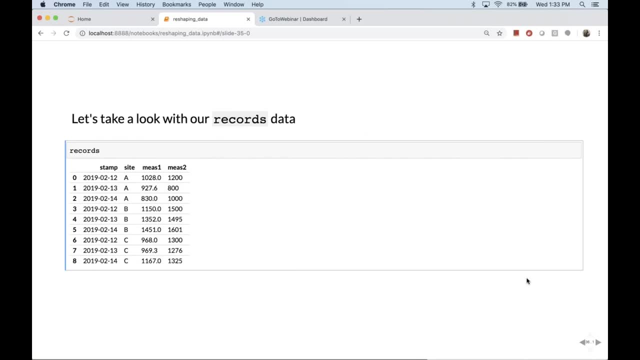 So let's go back to this records, data and look at it again. right, We've got some timestamps on the first column, We've got these sites in the second column and then we've got some numbers, measure one and measure two. 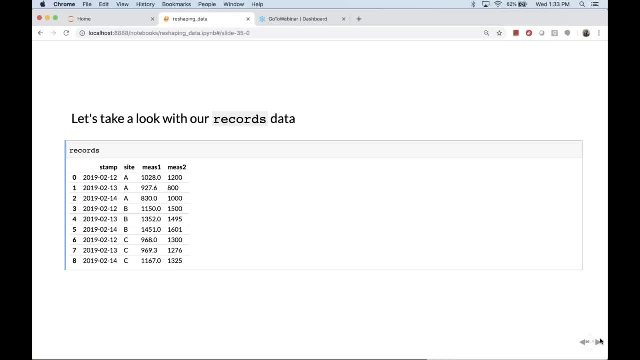 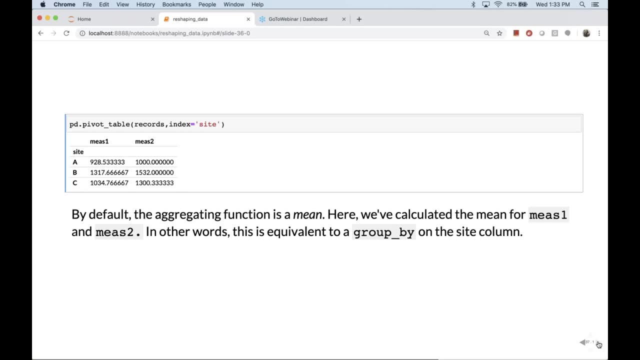 What can we do with this data with a pivot table? Well, we could pivot this data on the site index By default. our aggregating function here is a mean. So we've calculated the mean for measure one and measure two based on those different dates of the three sites here. 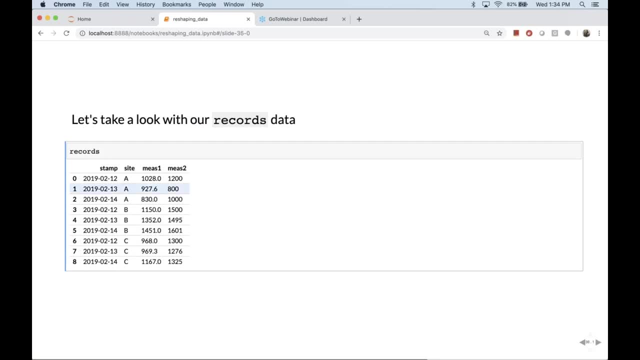 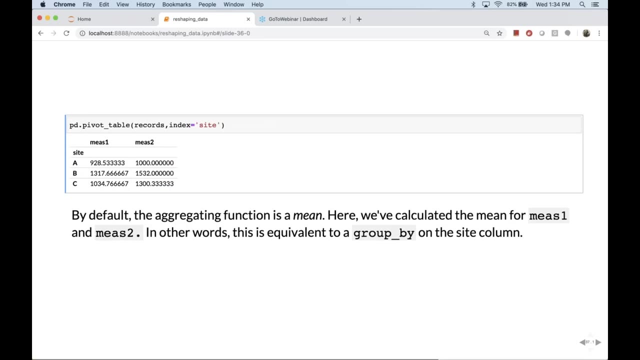 So, whatever these sites were on different dates, here with measure one and measure two, by using pivot table we've calculated the average value for measure one at site A and the average value for measure two at site B and C as well, right, In other words? 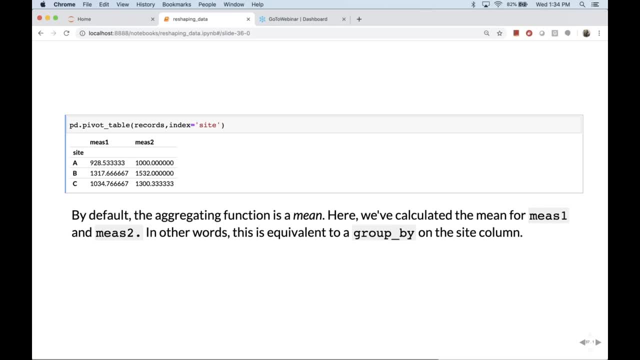 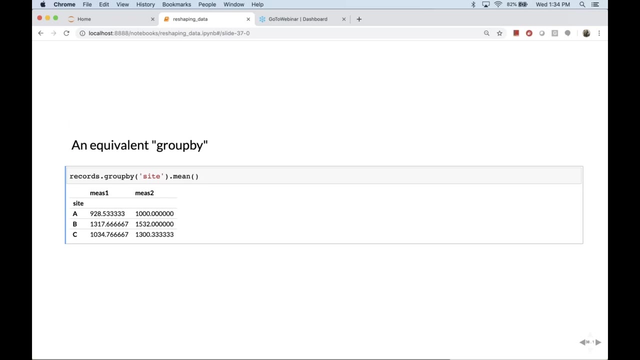 this use case of the pivot table is equivalent to the group by function. We could get these same results here by using Panda's group by function. So here's an example of that. We could have taken records We could have grouped on the site. 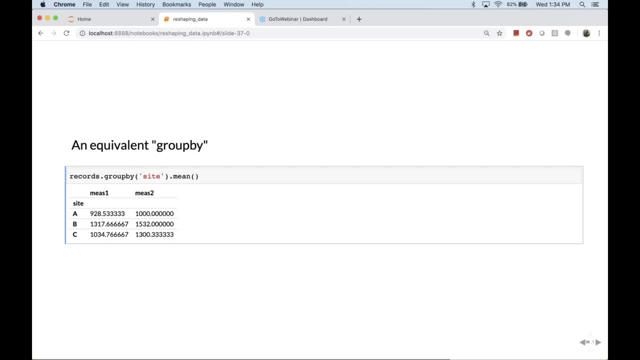 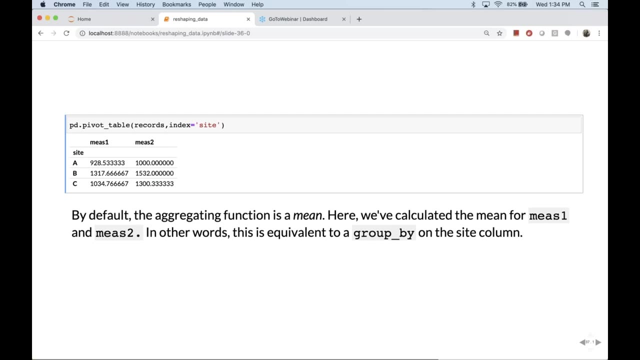 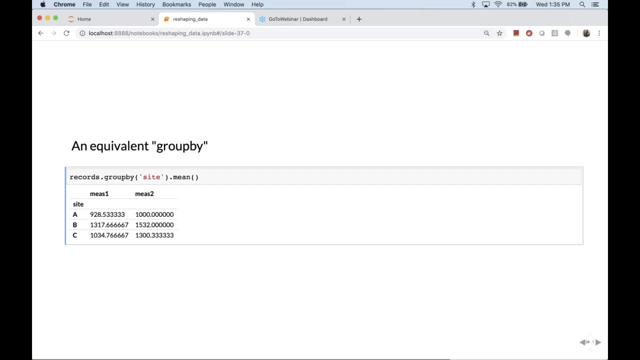 and calculated the mean and we get the same results as the pivot table. So that's the pivot table results. These are the group by results and they're equivalent. But pivot table has more tricks up its sleeve which we'll peek at now. 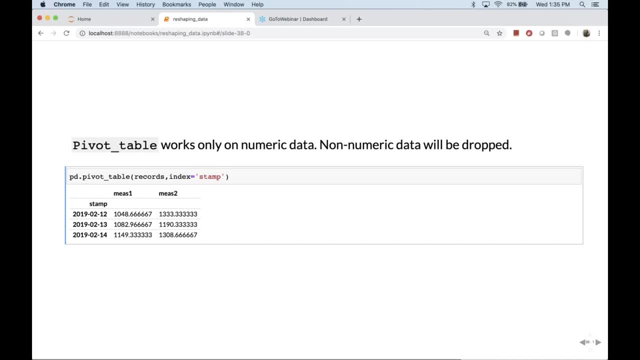 So pivot table is going to work only on numerical data. Non-numerical data is going to be dropped. So again, if we pivot on our records here with our index equal to those date times, we're going to drop the sites. We don't see the sites in the results here. 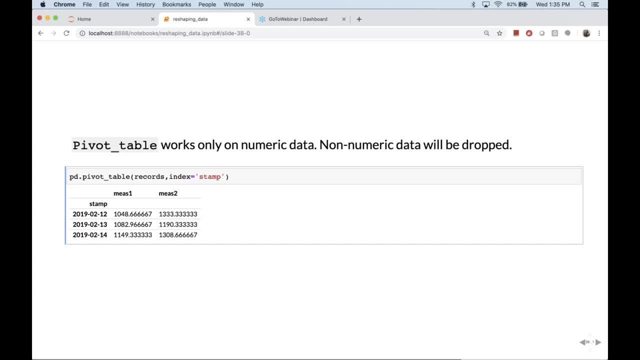 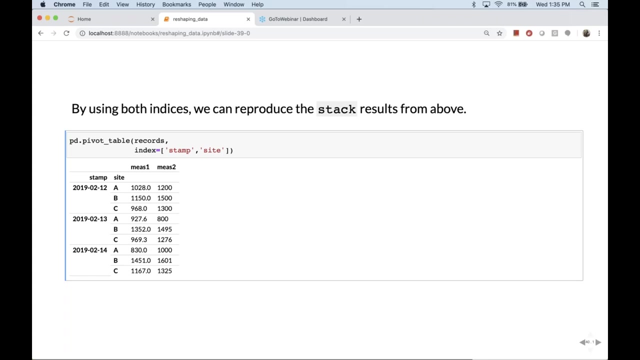 So we haven't told it to drop the site. but because we set the index to stamp we've pivoted the rest of the data set. It has dropped that categorical site column here If we use both indices here with pivot table, so stamp and site. 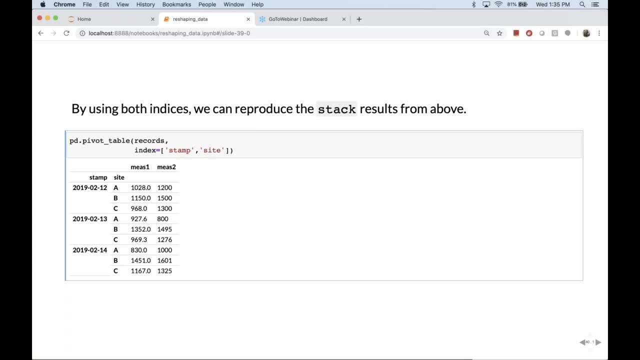 we're reproducing the stack results from above. So, again, what we're trying to illustrate here is that you can get to some of the same endpoints by using different methods. So there's always we're working with the flexibility of pandas and Python. 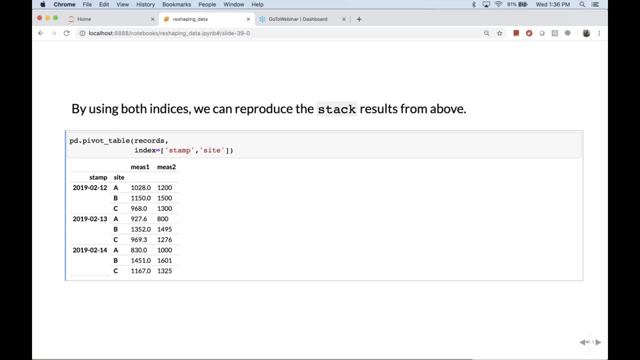 There's always more than one way to accomplish your goal. Pivot table will also can also create something like that stacked data result that you had above. Depends a little bit on what the underlying aggregating function is. Again, the default is the mean. 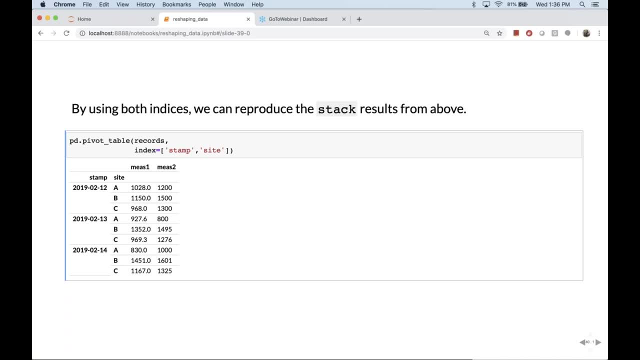 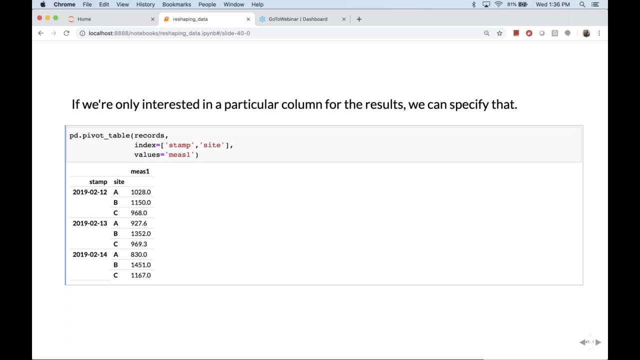 because we only have one record per stamp and site, we get equivalent results. That may not be the case In this example. it does give you the equivalent results to the stack method above, If you're only interested in a particular column in the output results. 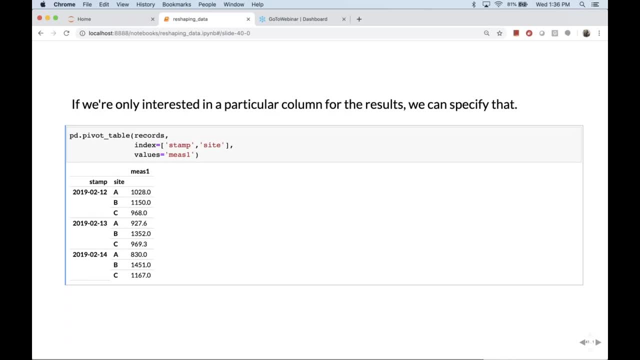 you can specify that with pivot table. So you can say: I want to take my data, I want to use these two indices As the new indices, hierarchical indices, on my output table. But I'm really only interested in measure one, I don't care about the other one. 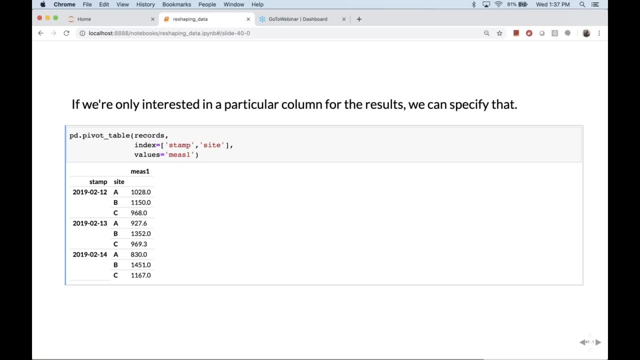 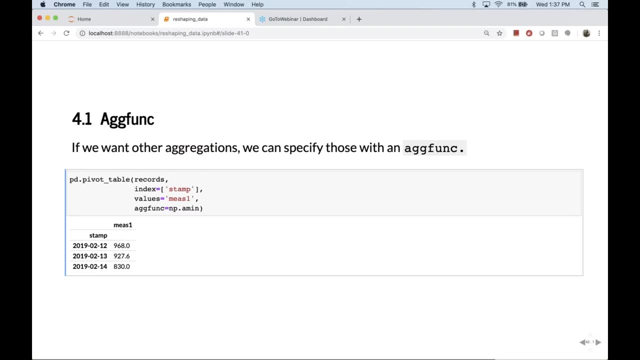 And I can subset the data down to that. Or- and this is the real power and flexibility of pivot table- You can specify other kinds of aggregating functions. So it takes a parameter which is the agfunk parameter, And that can let you. 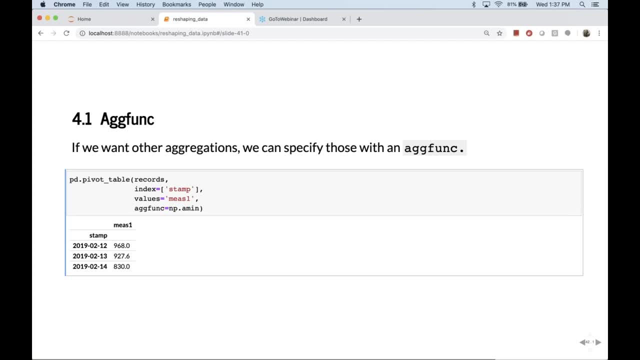 give you a lot of flexibility to do other kinds of table outputs here. So for instance in this example we could say: well, we want to aggregate on the timestamps, We're only interested in measure one, but we don't want the mean. 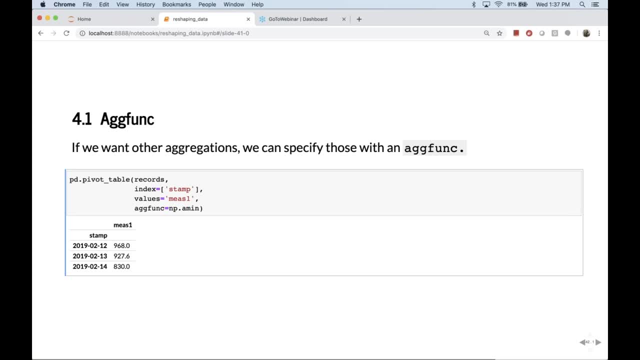 we want the minimum. So here we're using a numpy minimum function And you can use any numpy function that you want. in this You can use custom function that you've written. You can write a little lambda anonymous function in this slot here. 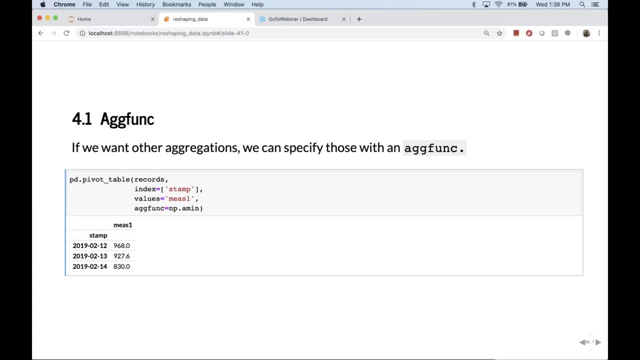 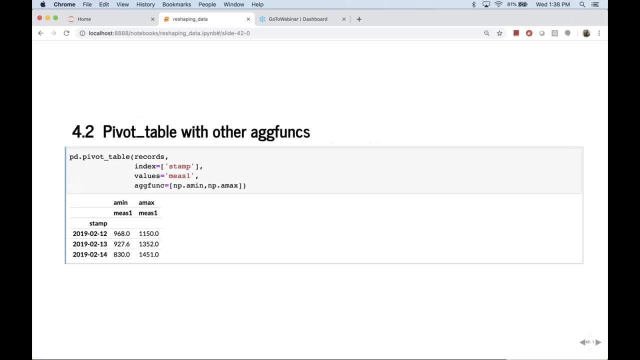 In this case we're using a numpy array minimum function to calculate those minimums. So what we have in the results are per date. per timestamp of the date, we have the minimum measure one in the results. Here's an example of using 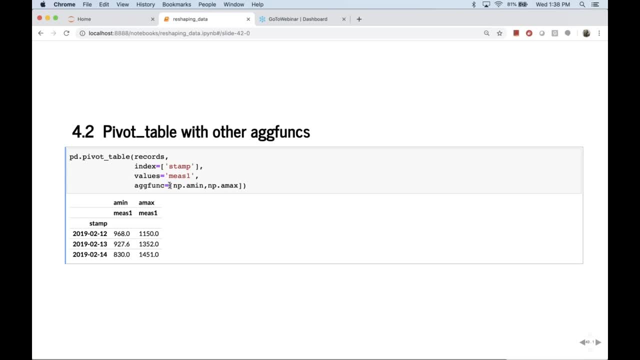 more than one aggregating function. So if we pass that as a list or list like object- here- and again we're using numpy functions- here min and max- numpy array min and array max- We can get this nice output that shows us: 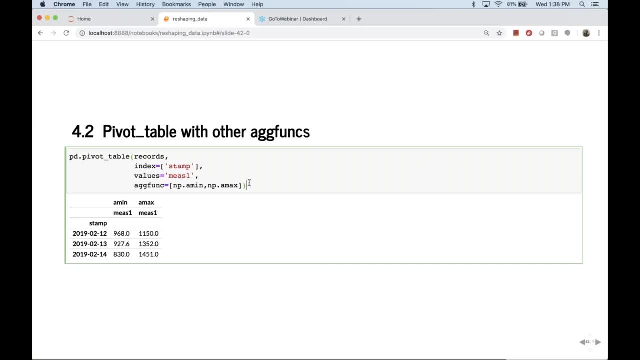 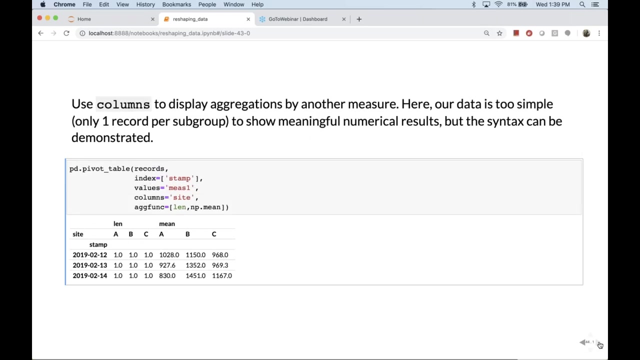 per date. for measure one, the minimum value and the maximum value, We can use another parameter called columns to display aggregations by another category. So here in this example we just want to stick with this data set and show the syntax. The data isn't too meaningful here. 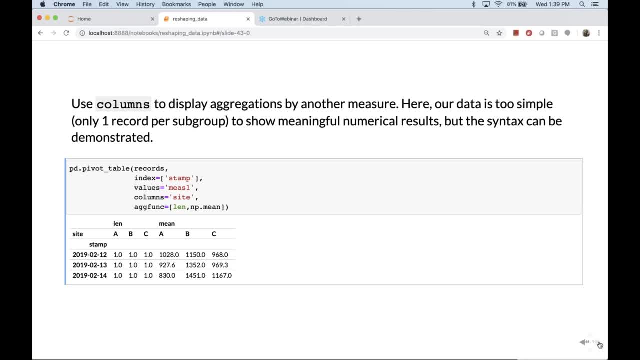 because we only have one Record per site and timestamp. but you get an idea of the kinds of tables that you can build here. And we're using two aggregating functions again, but instead of min and max we're using length L-E-N. 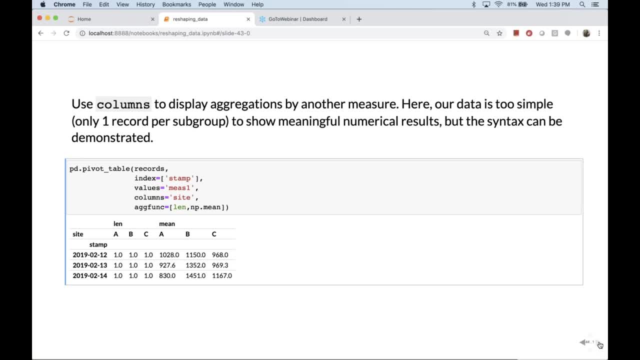 and that's going to be equivalent to a count. So how many records do we have at that timestamp per site A, B and C? So we've made a couple changes here. Again, it's that columns equals site to add this subgrouping here. 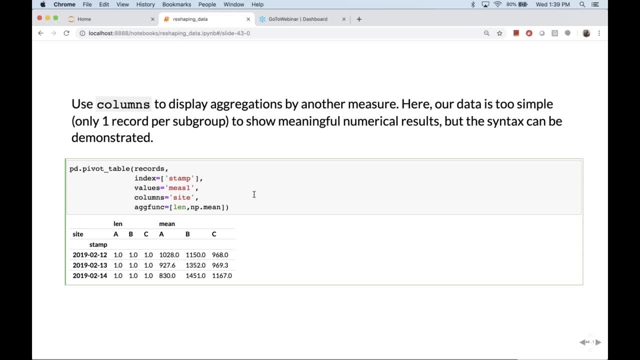 in the column indices And then just changing the aggregating functions to both length and the average, Again to get the average value per site and timestamp. So this is pivot table And again the idea here is that there's quite a bit of flexibility. 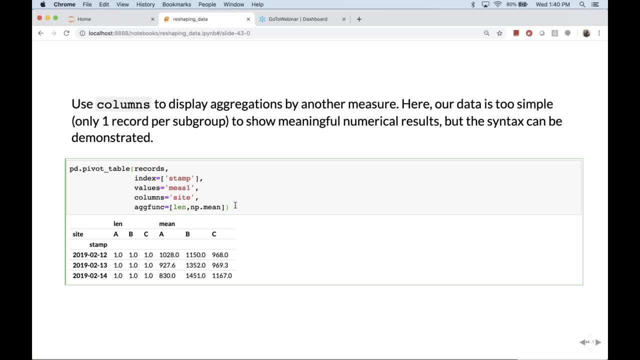 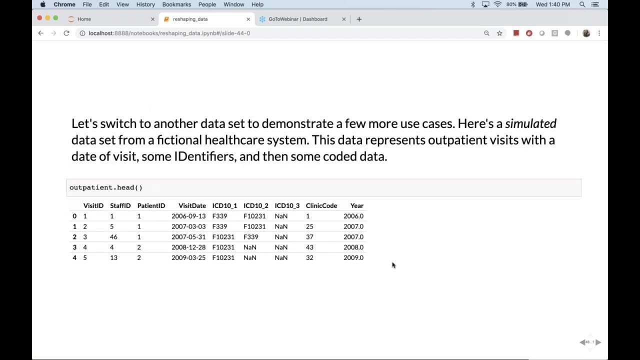 that it offers you, And the main power of it is this aggregating function and not only turning your data, but using these calculations As well. Here's a different data set that can illustrate some more of these use cases. So this is a simulated data set. 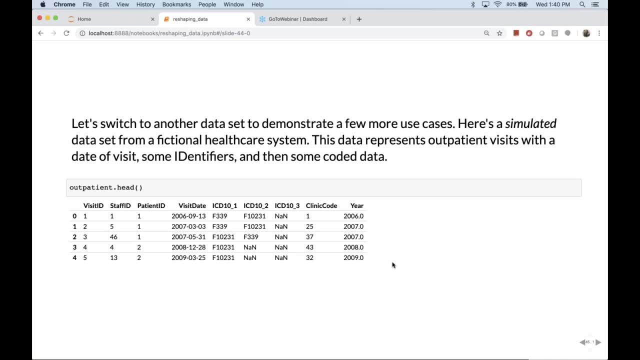 This is not real data from a fictional healthcare system, And this data represents some outpatient visits with a date of a visit, some identifiers, things like a visit ID, staff ID, patient ID- and then some coded data. So some diagnosis codes. 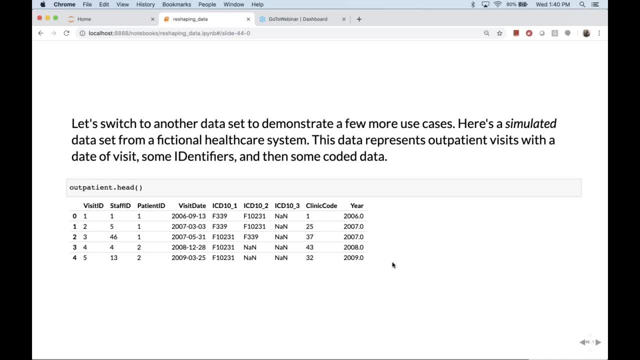 And we've created one more column here. We have the visit date, but we have another column which is the year just pulled out from that date. So we've got some identifiers, we've got some date data and then we've got some other coded data here. 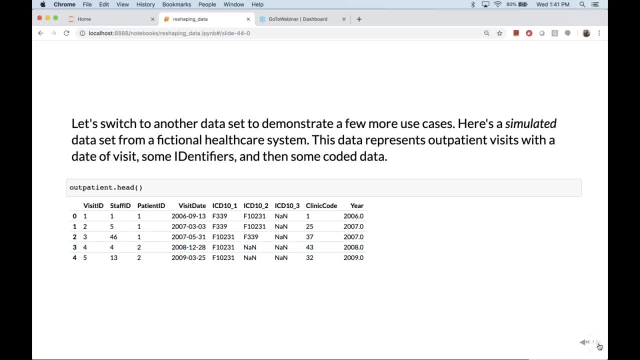 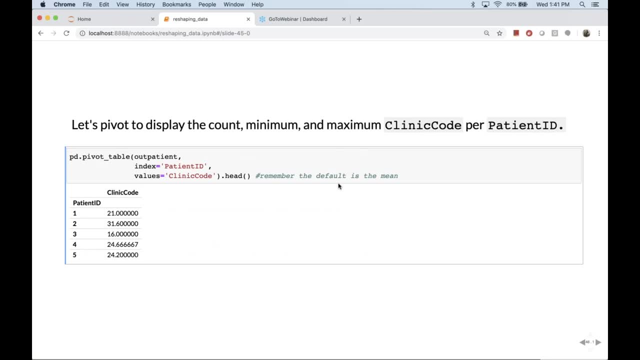 like clinic codes and some other diagnosis codes. Well, we can take that data, we can pivot it to display, for instance, the count minimum and maximum clinic code per patient ID. So here's one step along that path. We're taking the original data. 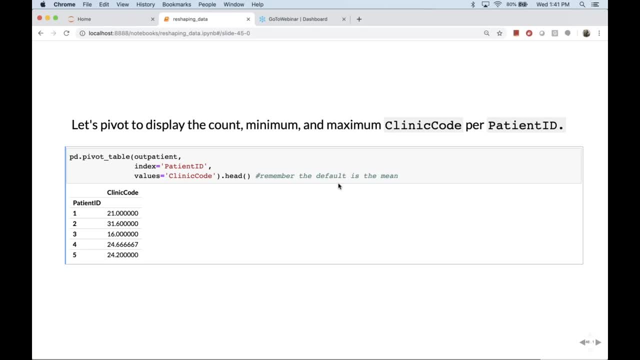 We're keeping our index as the patient ID and we're looking at the clinic code results as our values. Now, in this pivot, right now, what we're calculating by default? that aggregating function default is the mean. So this is the mean clinic code per patient. 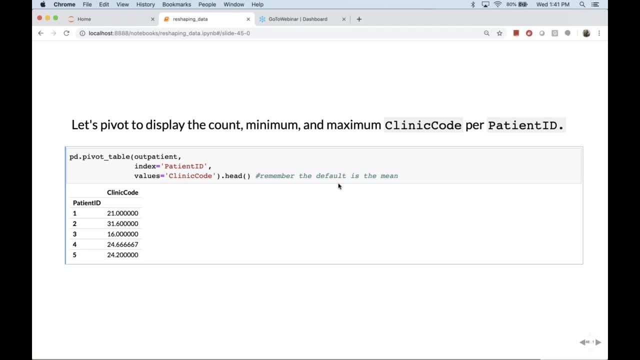 Again, maybe not so meaningful. We're just trying to display some of the syntax here, some of the way that pivot table works. So this is the average clinic code per patient if we go back to the original data here. So for patient one: 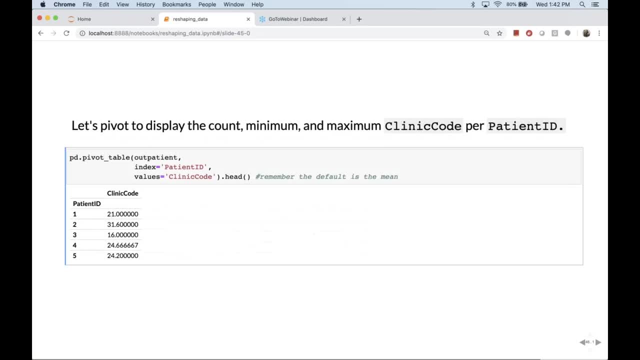 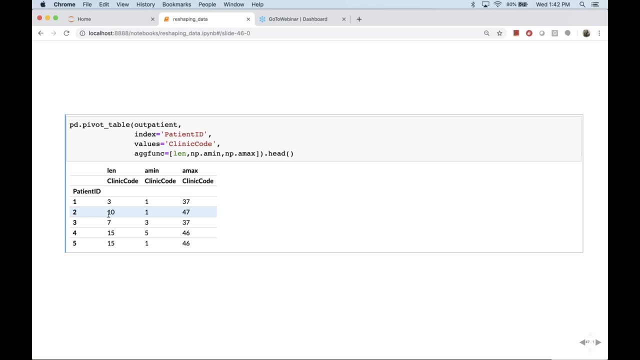 we had 1,, 25, and 37. The average clinic code for patient one is 21.. Again, not super meaningful, but just a display of the syntax here. Here this might be more useful data We can say. 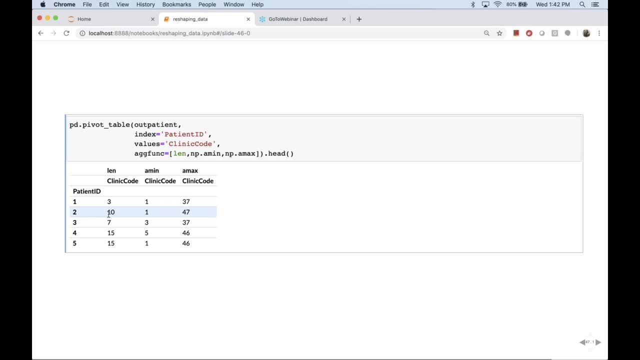 let's take the clinic codes by patient ID and instead calculate how many different clinic codes there are per patient. So again, that length function, that length function is going to be like a count function, And then we could use the min and the max. 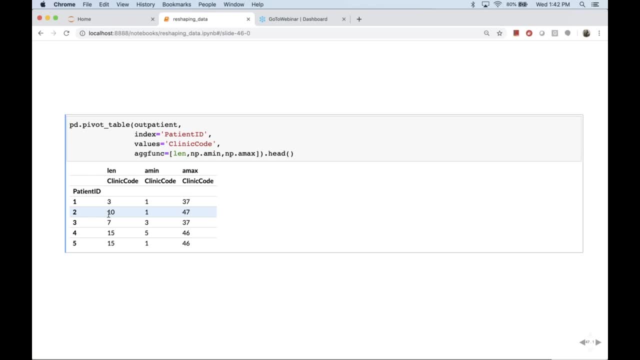 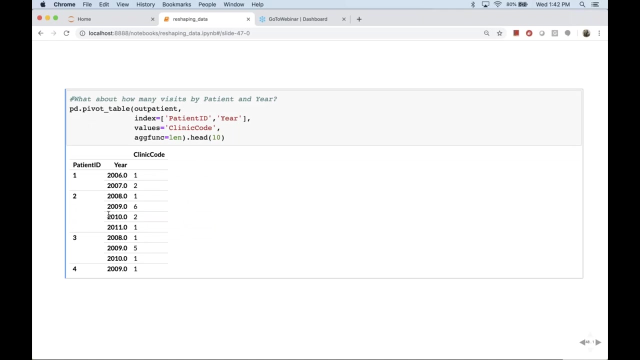 to get the smallest and largest clinic codes. Whatever it is that is useful for your rearrangement of the data. I'm just trying to use some other data here to illustrate some of this pivot table syntax. Here's another way that we could rearrange this data. 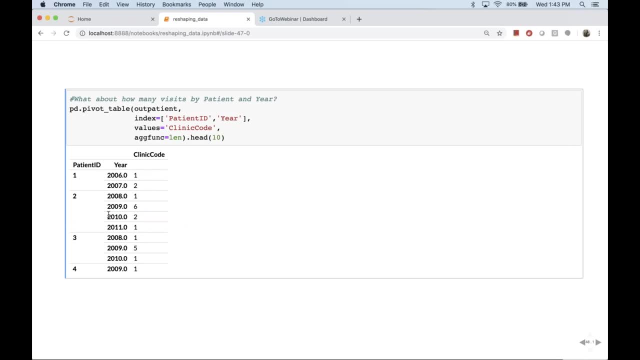 So we could use pivot table to say how many visits by patient and year. So we could count the clinic codes, the number of clinic codes, by two indices here, the patient ID and the year right, And that'll give us a count of how many visits there were. 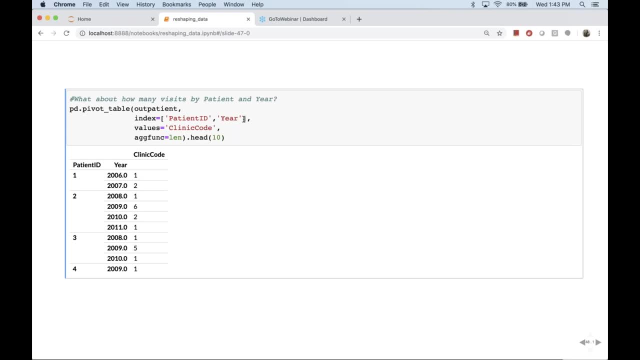 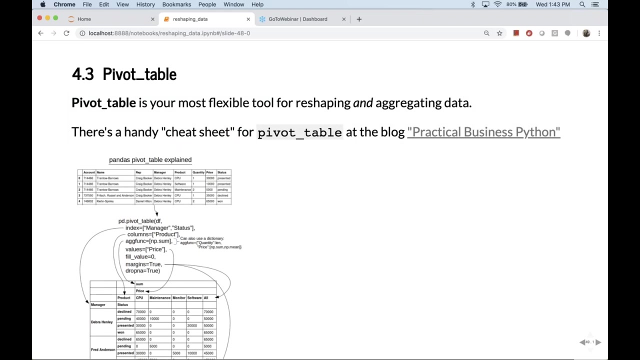 per patient and year. So we can see, for patient one, for patient two, the different years, the different number of visits. So pivot table is really your most flexible tool for reshaping and aggregating data And there's a handy cheat sheet out there on the web. 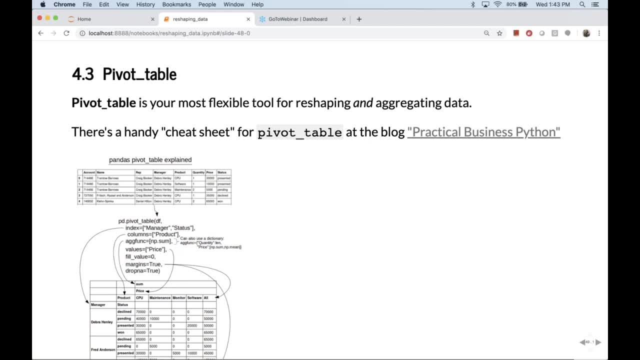 So there's a blog called Practical Business Python, and this graphic is taken from there. I really like cheat sheets and this is a great cheat sheet, So this is going to show you those in the center of this page. here, This is going to show you the syntax for the pivot table. 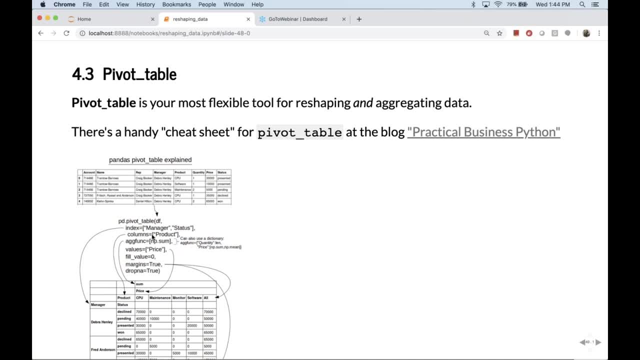 So your original data index columns aggregating functions and your values. There's some other pieces to pivot table here for you to discover, So things like filling in values. If you have missing values, you can give those a zero value Or a negative 999 or whatever makes sense for your data. 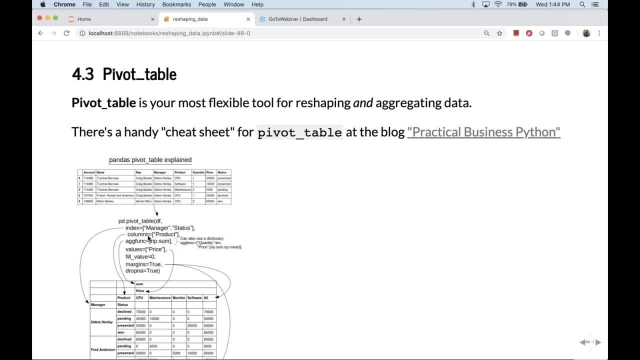 You can add margins to your output data tables. This is a great blog article. So if you again, if you look at Practical Business Python, this is going to run you through lots of functionality for pivot table to show you lots of different ways. 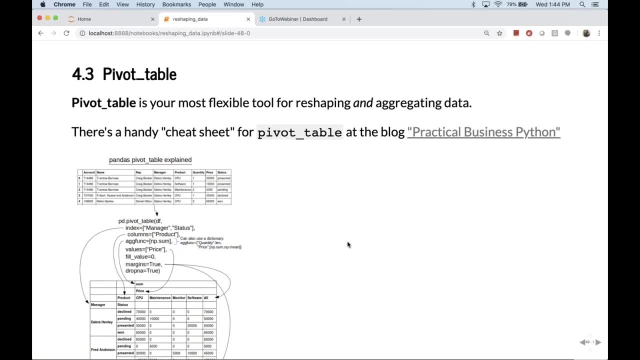 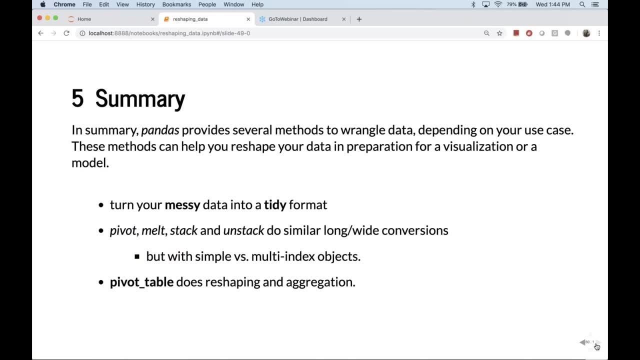 that it can be used and maybe spark some ideas for you to use it in your own workflow. So, in summary- and then I'll answer some questions here, if there are any- Pandas is going to provide you several different methods to wrangle your data, depending on your use case. 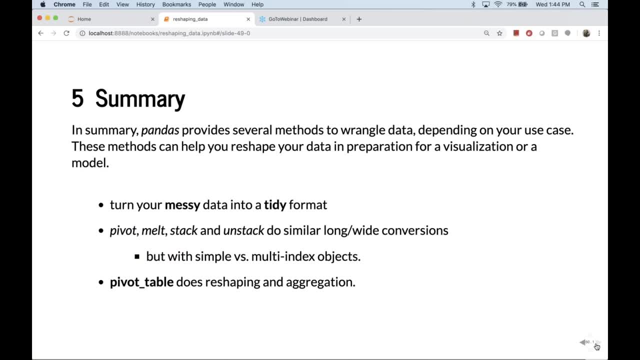 These methods can help you reshape your data in preparation for a visualization or a model. When do you want to do this? Why do you want to do this? Well, in general, if you're not sure where to go with your data, try to think about turning your data from a messy format. 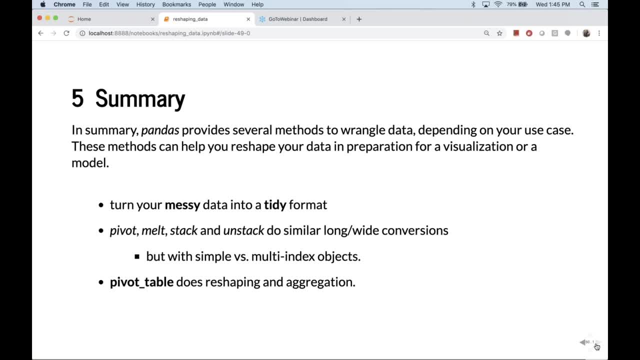 into a tidy format, So that can be one move off the bat that you can do if you're not quite sure where you're going to go with your data, What you're going to do with your data Otherwise, our recommendation would be to reshape it depending. 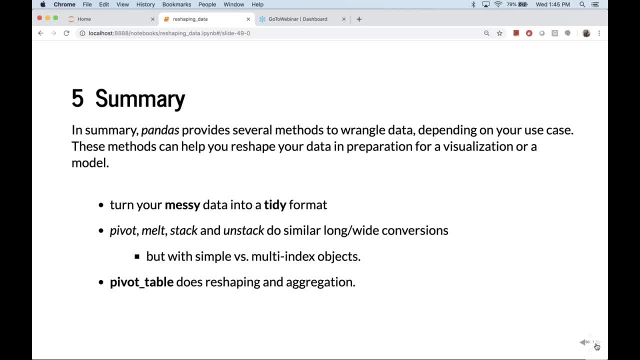 on what you need to do with your data. So are you doing a presentation, Are you doing a visualization, And what are those variables that you need in the output results? That's really going to help you guide you to what kind of methods you need to use where you're going to. 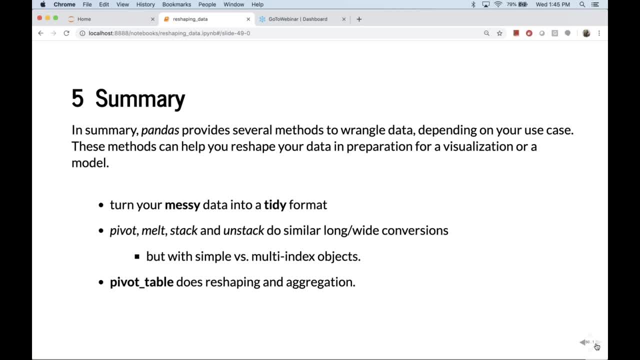 So take a moment to write down what variables you need to look at. Those are the ones that you want to put into columns And that should give you a starting point for reshaping your data. What methods do you use to reshape this data? 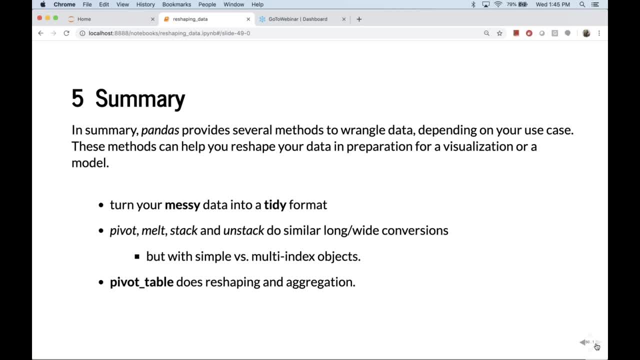 Well, the pivot, melt, the stack and the unstack all do similar long and wide conversions. But the difference here is really: are they taking simple or multi-indexed objects? Stack and unstack are those ones that will take multi-indexed objects. 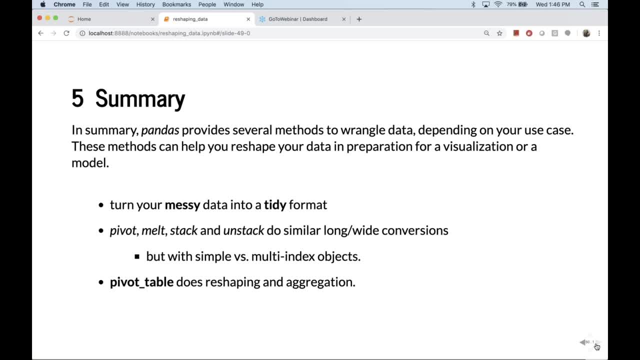 Pivot and melt are more flexible. They have a lot more parameters to them, but they expect more simply indexed objects, although they can result in multi-indexed objects in the output. Pivot table is the overarching one that does that reshaping, but with aggregation. 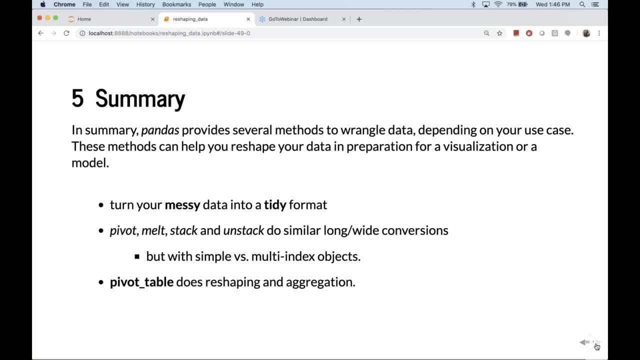 So if you need to do some recalculations, if you need to do means counts, minimums, maximums, sums, things like that, that's when you're probably going to reach for pivot table if you want to do that, reshaping and aggregation. 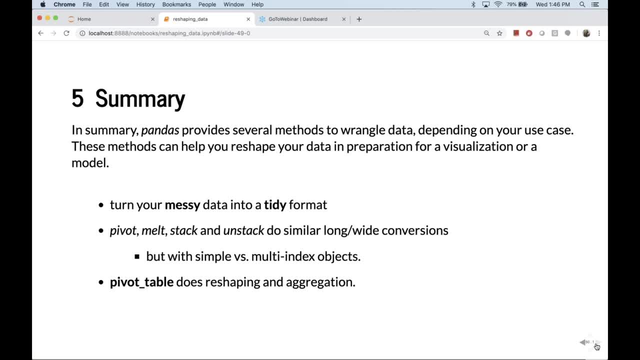 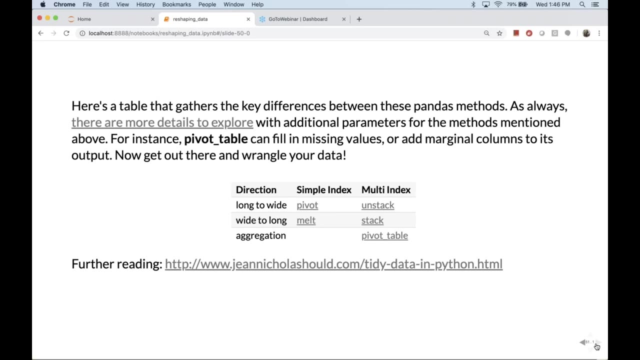 In other words, if you have more than one record in the output, potentially more than one record in the output- you're going to need to do some kind of pivot table methodology on it. So again, here's that same one I just talked about as a table. 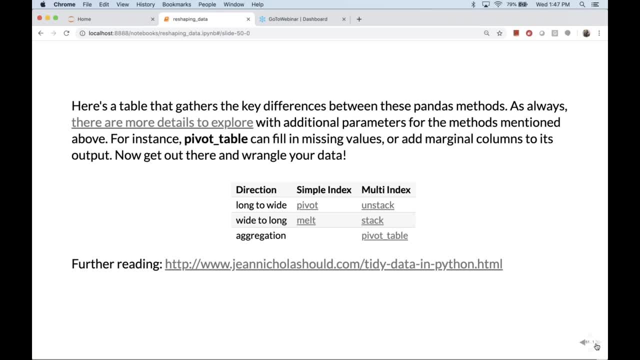 You can look over. There's more details. We've covered most of what pivot and melt and stack and unstack have to offer, but always check the Pandas documentation for more details about it, and there's a nice article on Pandas as well that covers some of these toy cases. 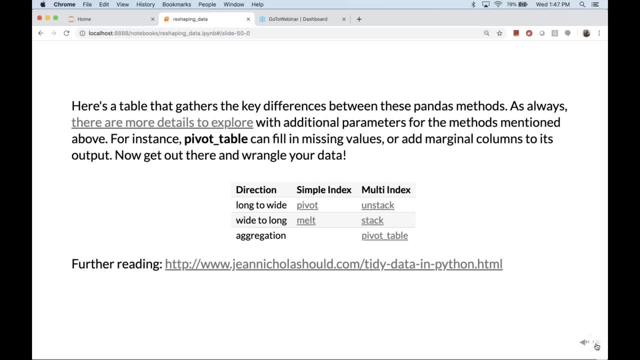 some of the things that we've talked about here. This is a really nice article as well. This is just a blog post here that talks about the idea of tidy data in Python and it's going to run you through some use cases, So this is inspired again by the R idea of tidy data. 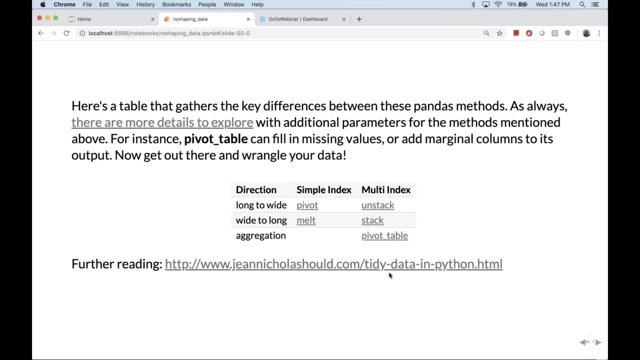 and this link down at the bottom: tidy data in Python. if you do a search for it, it should come up. That's going to run you through different kinds of data formats and show you how to use Python and Pandas- the same methods that we've shown here. 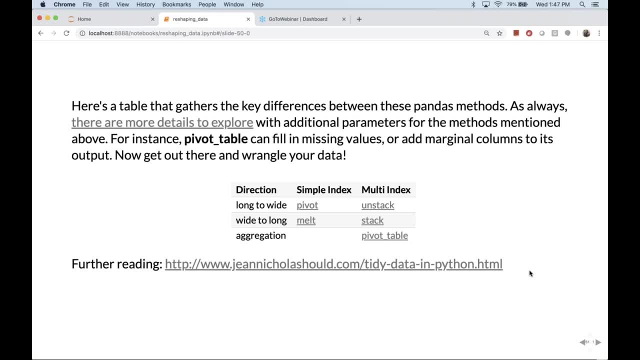 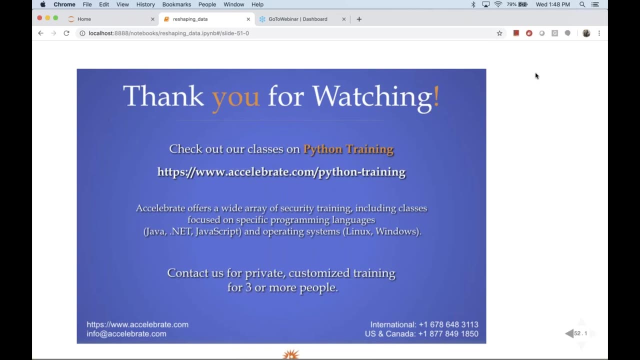 how to use them to move data from any messy format- different kinds of messy formats- into a tidy format. Great. so thanks so much for watching. That's our webinar on Pandas and reshaping data with Pandas. I'll hang out here online and, if you have any questions, 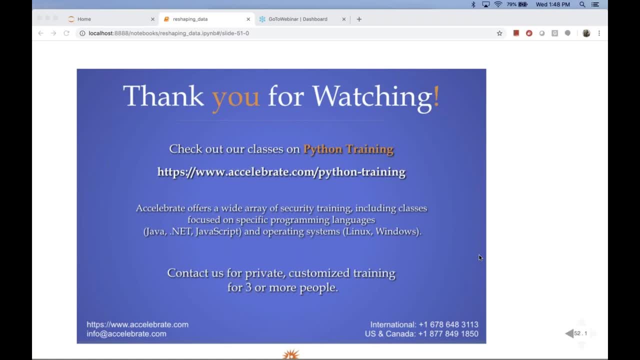 feel free to send them to me in chat or to post a question, and I'm happy to try to answer that if I can. I think one of the challenges with reshaping data is that- and there's a quote that the R authors of the Philosophers of Tidy Data. 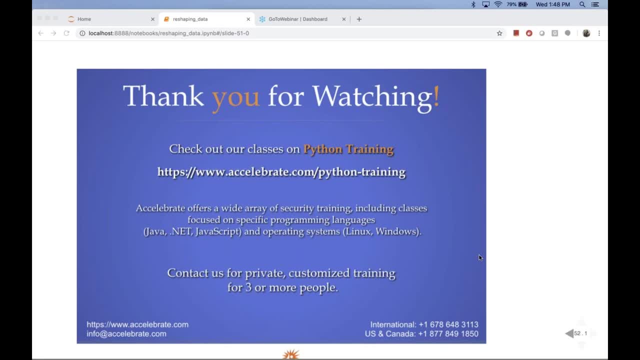 have talked about is that tidy data again tries to be this idea of consistent format. Messy data tends to be messy in lots of different kinds of ways, So beyond this, it's hard to make consistent rules and say: go from. 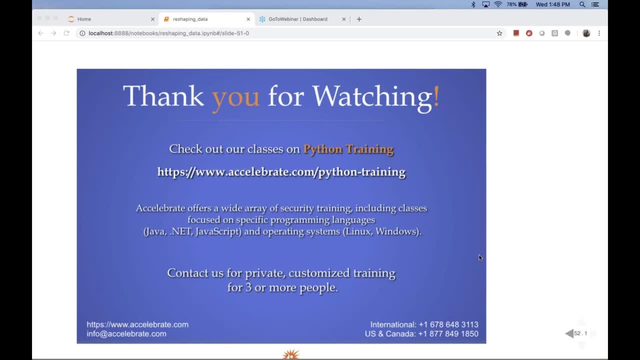 you know, always put your columns in this kind of format, always put your dates in this kind of format. We really need different solutions depending on what the incoming messy situation is, But the idea of tidy data can really help, sort of direct you. 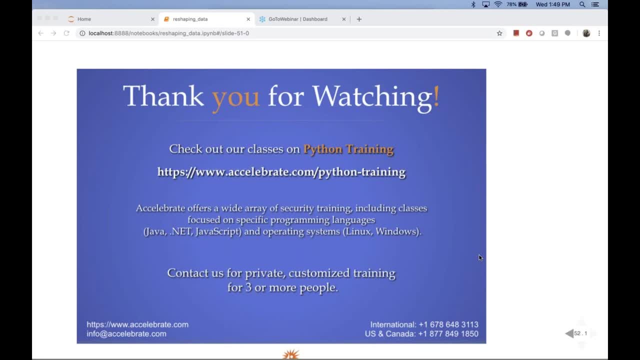 if you're not sure where to go, and the guiding principle for you should really be: what do you need to do with your data? What do you need to accomplish with it? Are you trying to present it to an audience? That will guide what kind of format you need to take your data in. 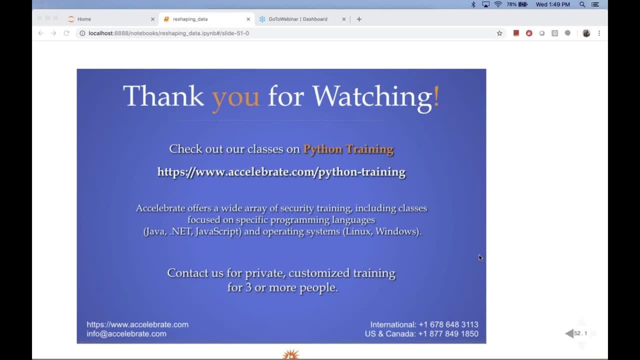 And then what we've discussed here with different methods are the ways that you can accomplish that. So thanks so much for attending this webinar And again, I'll hang out here for a few minutes and take some questions. Feel free to chat me any questions you have and let us know if you have any.